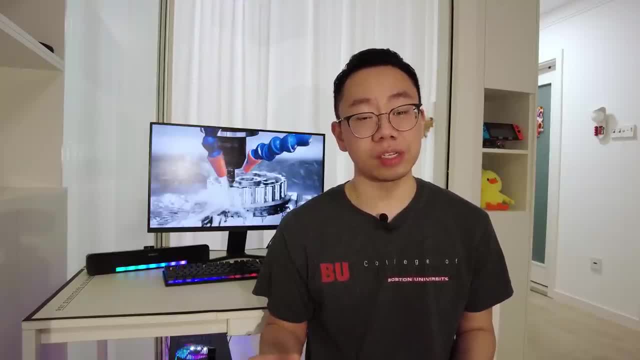 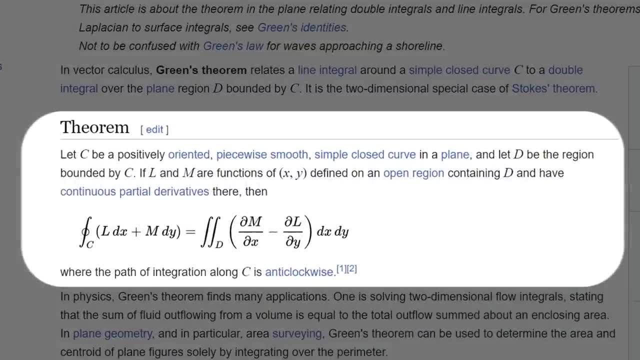 that the bodies of knowledge you need to land your dream engineering job. I want to emphasize here that the bodies of knowledge you need to land your dream engineering job. I want to emphasize here. But these are actually covers all about how students can beautifully Siberian. 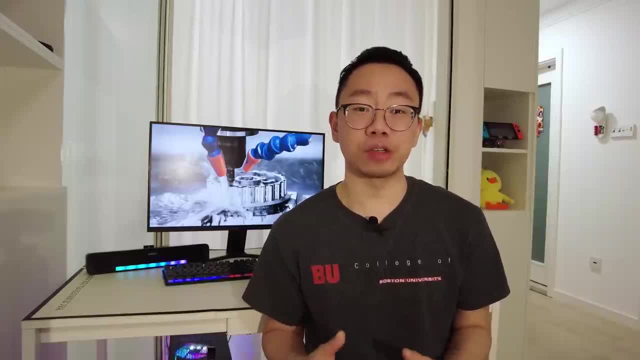 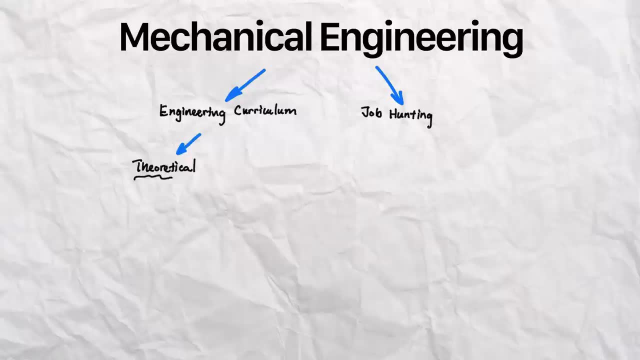 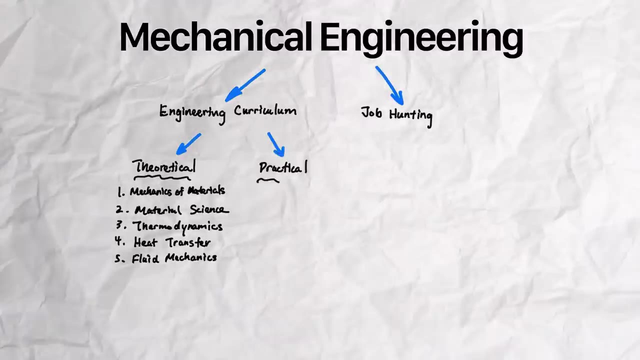 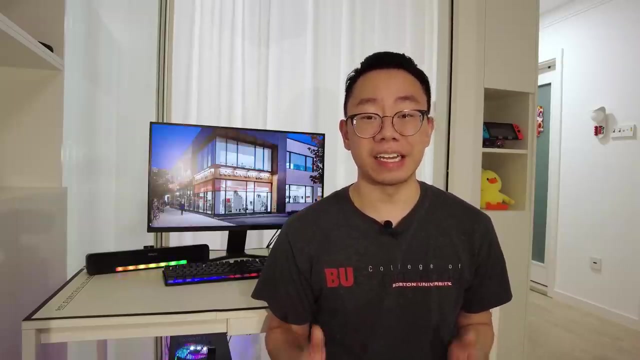 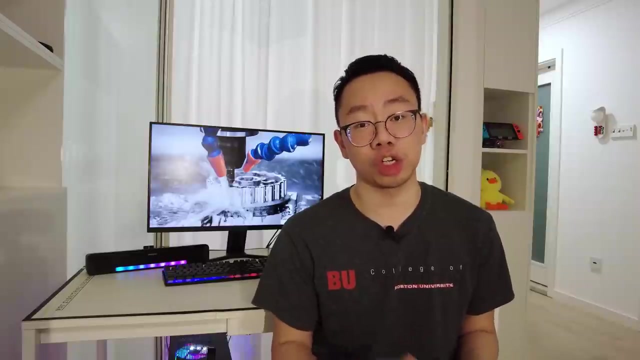 be qualified in the module class for engineering job interviews. or yuan нhe 回过 comings stereo result 实adas taught in these classes is important because it's fundamental knowledge that every mechanical engineer who designs products and processes should know and will help you pass more engineering. 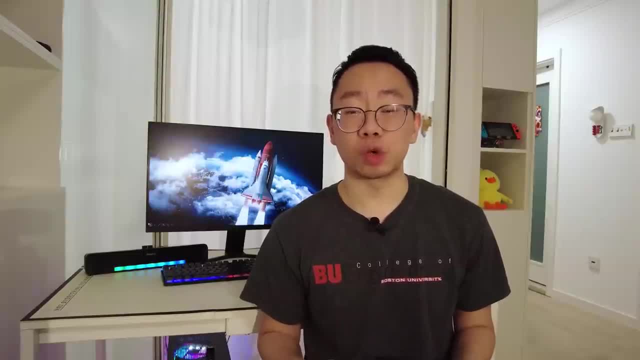 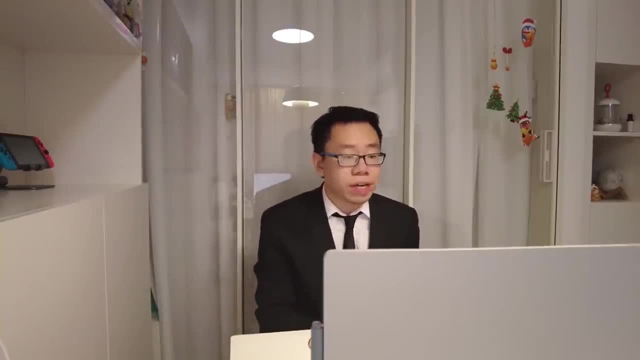 interviews. Now, while having this fundamental knowledge is a great starting point, it doesn't really guarantee you'll get your dream job, because you really never know what the interviewer is going to ask. So later in this video I'll talk more about this and how you can pass more engineering. 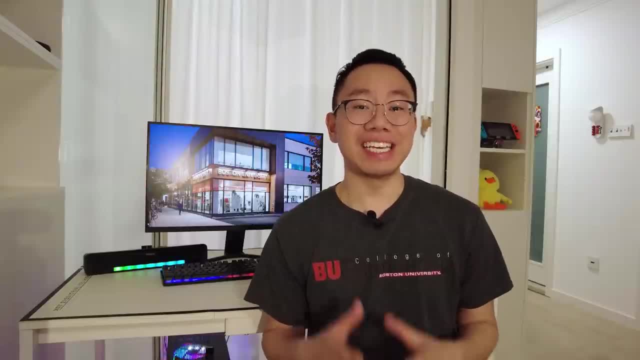 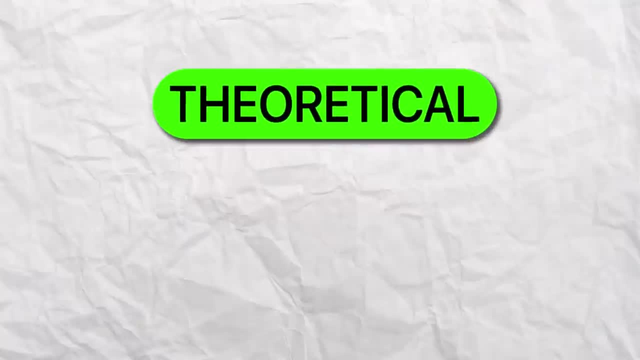 interviews in general. So let's begin by talking about the essential engineering topics that are commonly asked in job interviews and that you should focus on as a student. We'll start with the theoretical classes, the first being material science- Important topics that you should know. 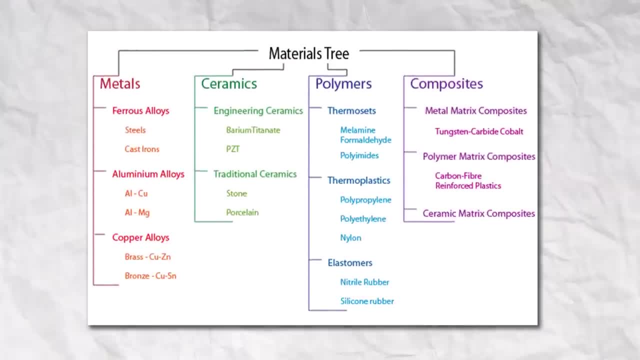 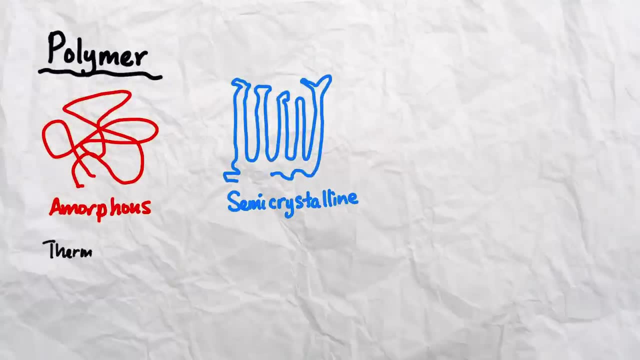 include the structure and properties of materials, including metals, polymers, ceramics and composites. For example, the structure of polymers is either amorphous or semi-crystalline. Thermoplastic polymers can be melted and reused, while thermostats 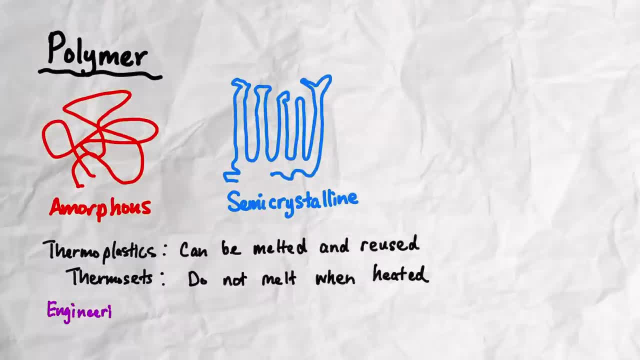 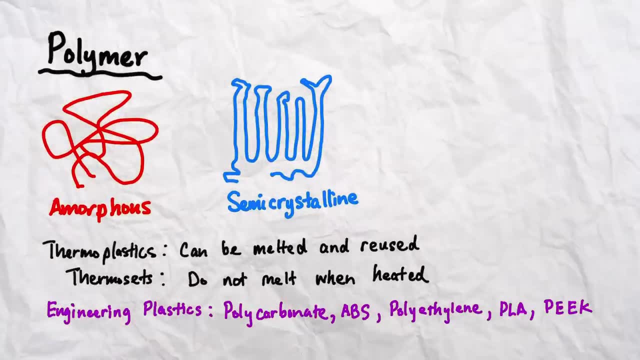 polymers do not melt when heated. You should also be familiar with different types of engineering plastics, such as polycarbonate, ABS, polyethylene, PLA and peak. Expect to be asked about some of these materials in a job interview, including their material properties and applications. 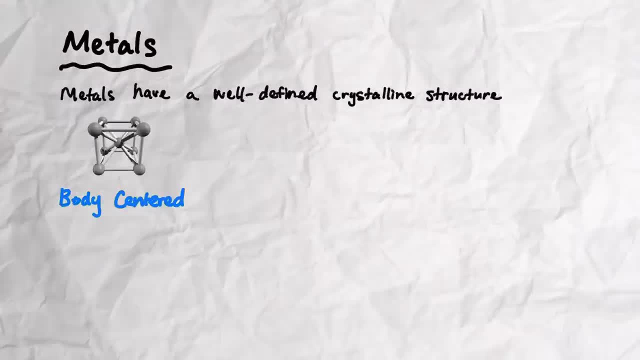 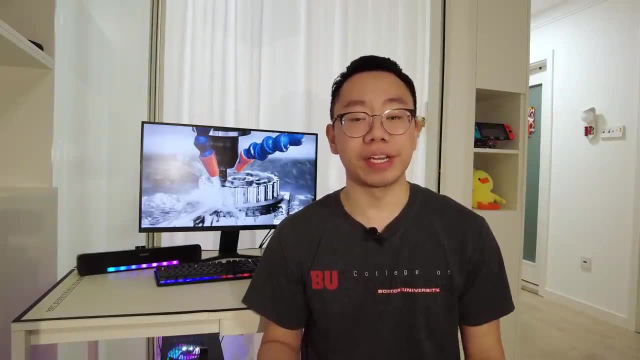 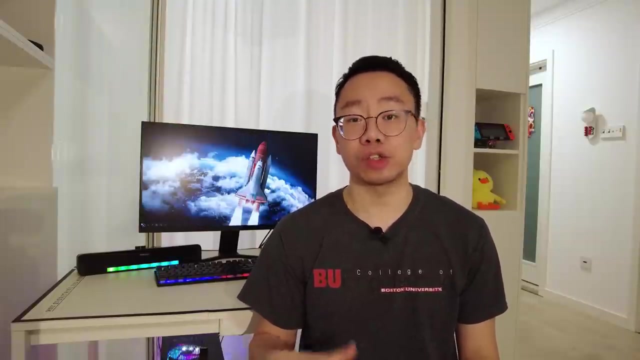 Metals, on the other hand, have a more well-defined crystalline structure, including body-centered cubic, face-centered cubic and hexagonal closed path. When it comes to metals, you should be familiar with the various types of heat treatments and strength strengthening mechanisms used to enhance their mechanical and chemical properties, such as strength. 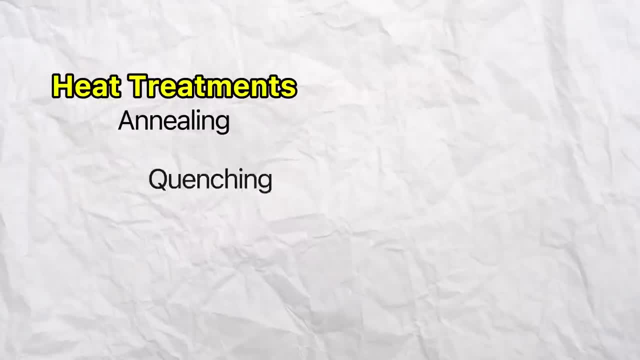 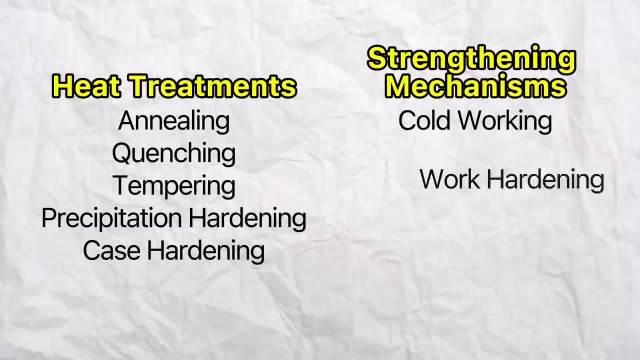 and hardness. Common heat treatment techniques include annealing, quenching, tempering and precipitation and case hardening. Strengthening mechanisms at room temperature include cold working, work hardening and grain boundary strengthening. A phase diagram is often used. 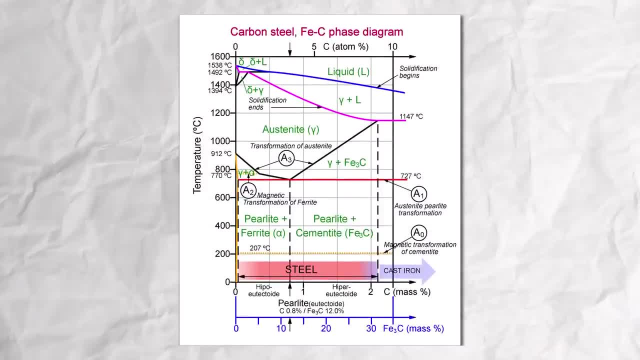 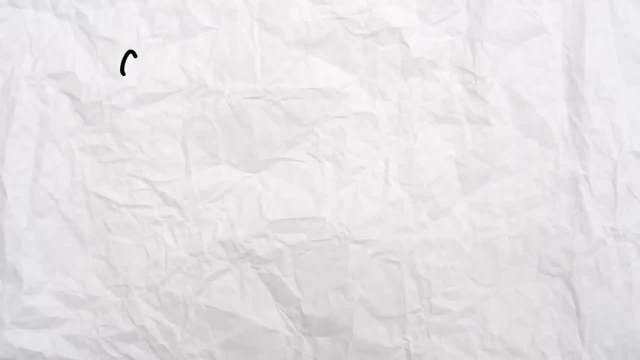 by material engineers to understand how metals and plastics behave at different temperatures and pressures. Composites, on the other hand, are made by combining two or more materials. There are metal matrix composites, plastic matrix composites and ceramic matrix composites. 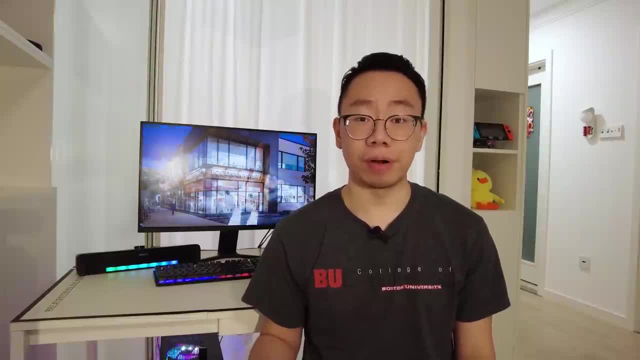 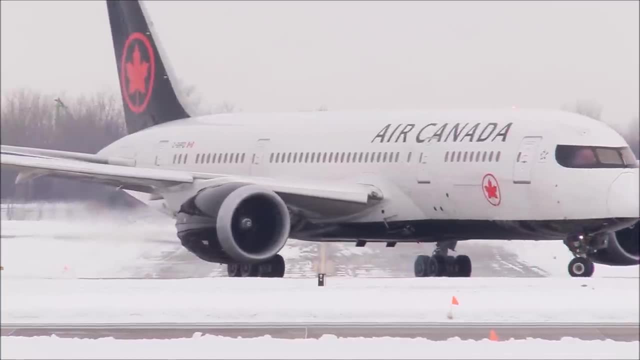 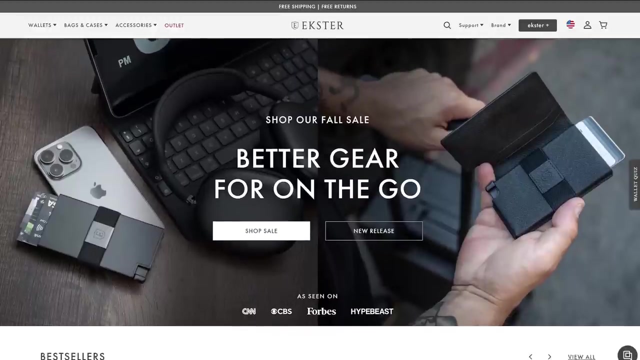 The most popular composite is probably carbon fiber, which offers superior strength, durability and lightweight properties. They're used in automotive and aircraft components, as well as this fancy, stylish wallet by Ekster, the sponsor of today's video. Ekster is the leading maker of 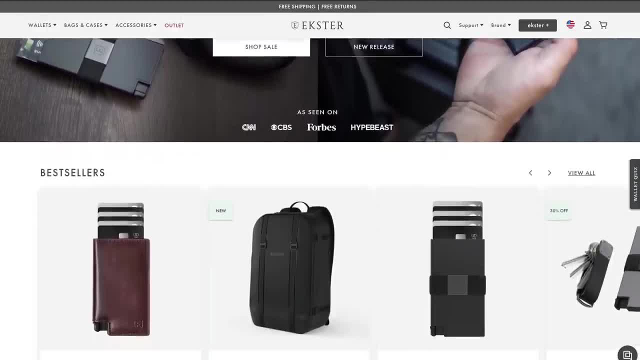 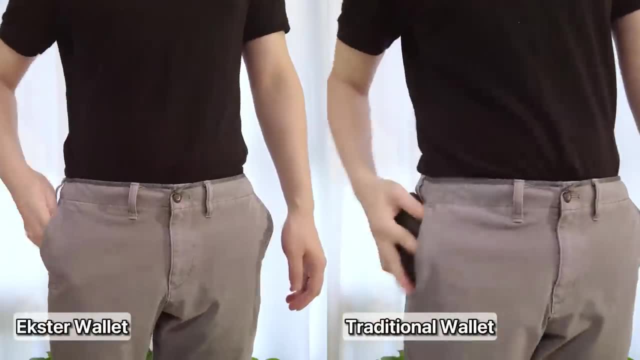 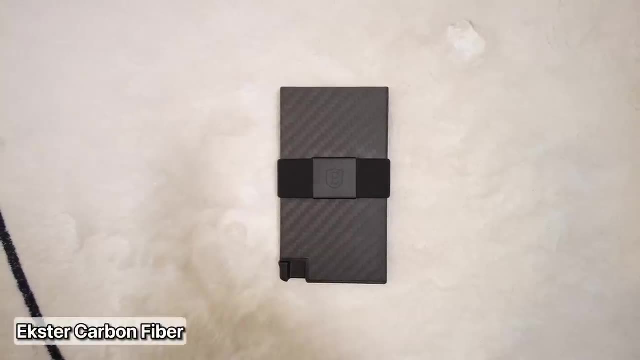 smart, minimalist wallets offering top-notch quality, a futuristic design and cutting-edge RFID blocking technology. Ekster wallets are ultra slim, freeing you from the burden of traditional bulky wallets, and come in a wide variety of colorways and materials. One of my favorites is their carbon fiber wallet made from 3K space-grade carbon fiber. 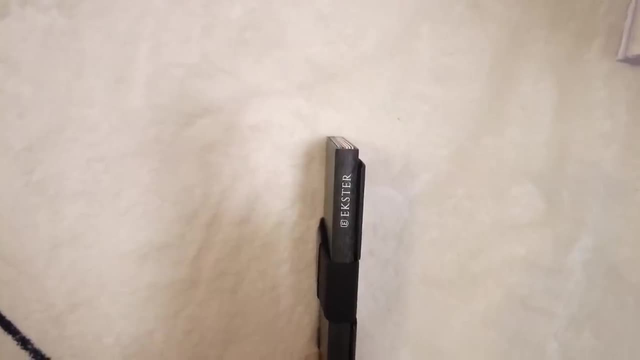 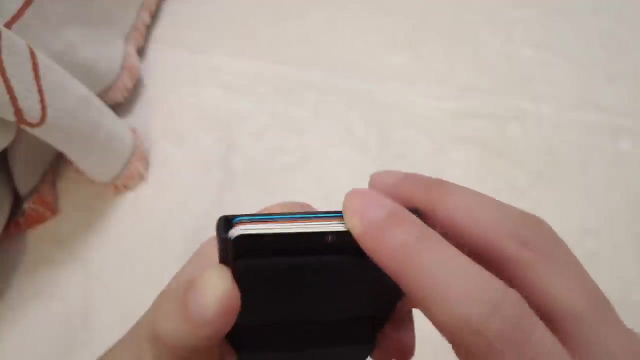 commonly used in aircraft fuselages, so the wallet is extremely light and will last for ages. You can fit up to 6 cards in this slot and additional 6 cards in this backplate, for a total of 12 cards. You can also hold your cash in this slot, which is great for your cash and 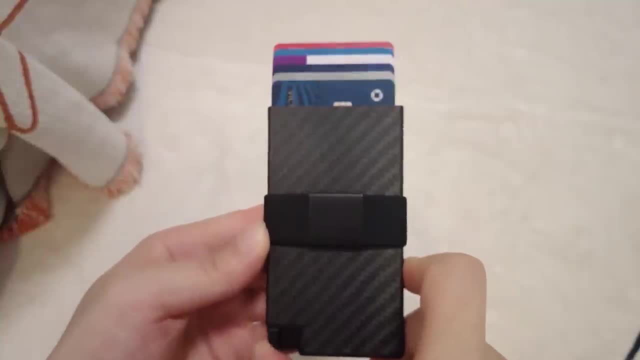 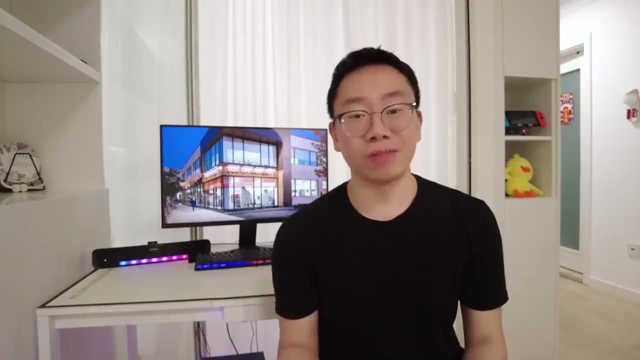 in the front with the rubber band. all of extras. wallets feature a trigger mechanism at the bottom for easy access, so you're always ready to pay, no matter how fast life moves. if you're a fan of letter wallets, extras got you covered. this is the parliament, which is extra stylish flagship wallet. 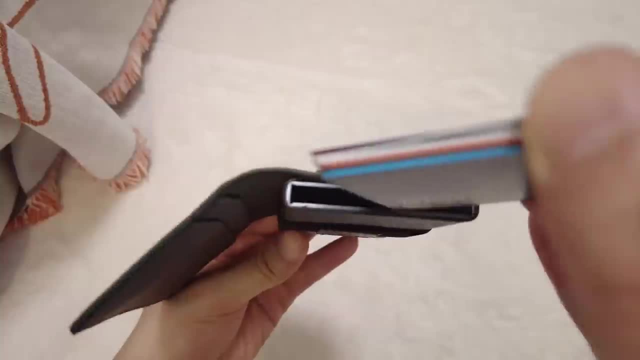 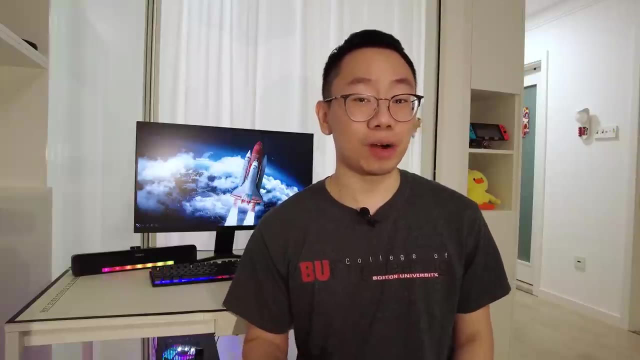 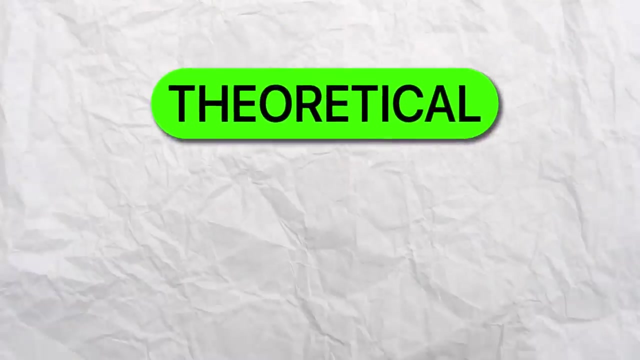 made from premium, environmentally friendly leather that features an aluminum card holder and can hold up to 12 cards. i partnered with extra to give you guys an exclusive discount. get 25 off now through my personal link or code egw, listed in the description below. let's move on to the next class. 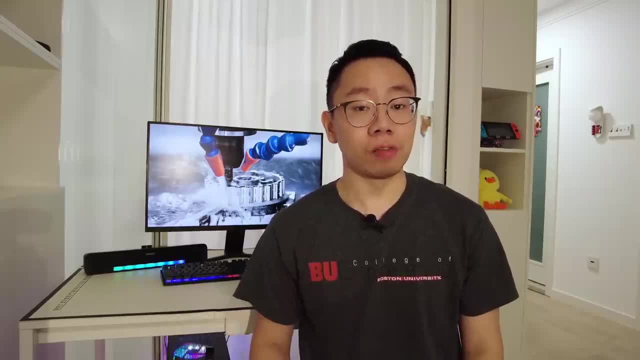 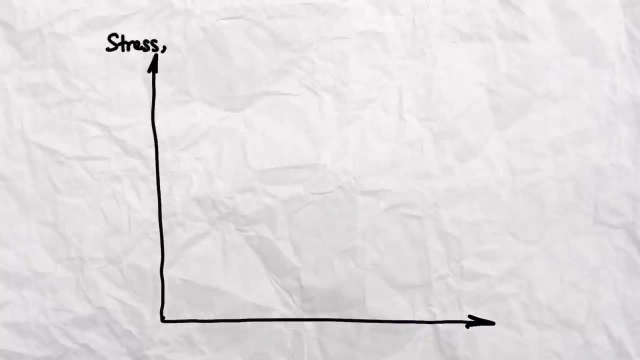 mechanics of materials. one of the most important topics covered in this class is the stress strain curve. this is a graph that shows the relationship between stress applied to a given material on the y-axis and the resulting strain it undergoes on the x-axis. stress is a measure of how much force. 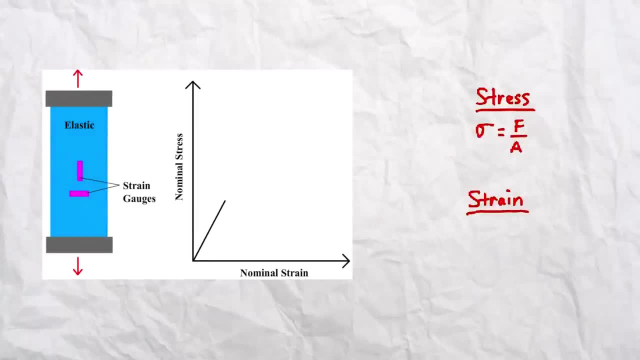 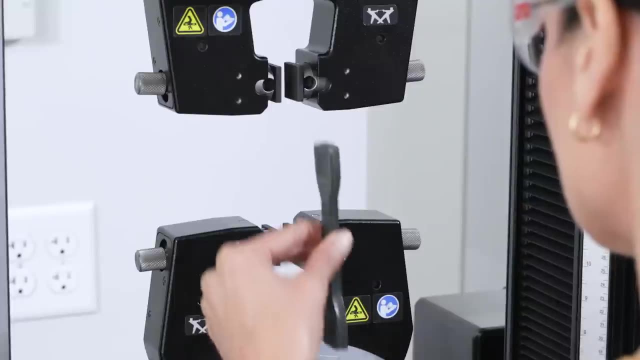 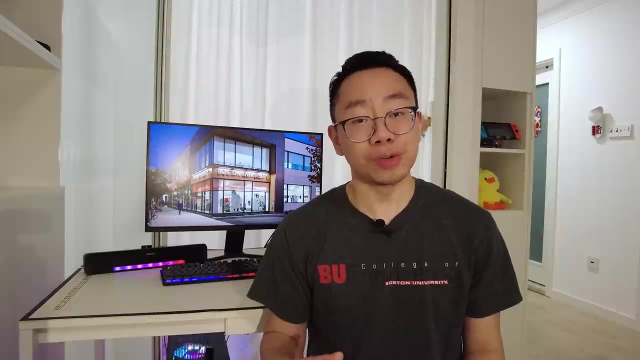 that's being applied per unit area, while strain is the amount of deformation the material undergoes when subjected to stress. this graph will look different for each material and is obtained by stretching or compressing a piece of material in the shape of a dog bone on a universal testing machine. engineers use these. 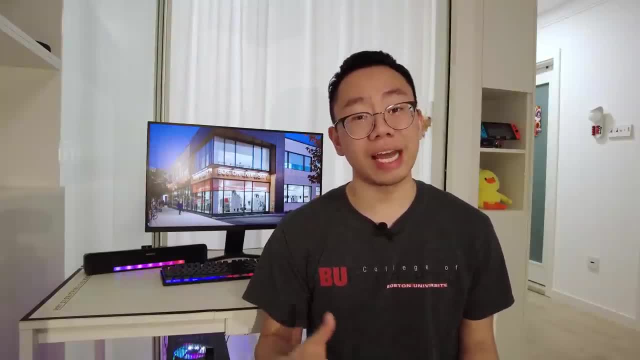 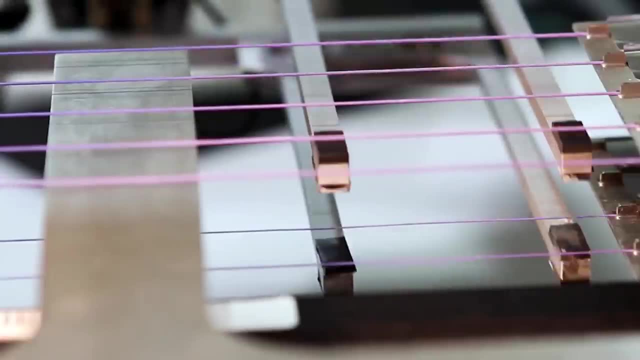 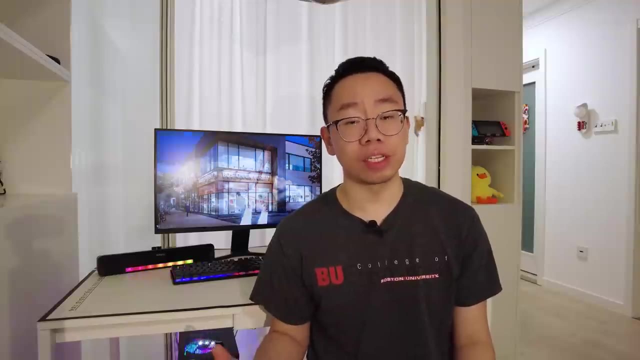 curves to select materials for a new product to ensure that it can withstand the mechanical forces that it will encounter in its end-use application. for example, surgical sutures must have enough strength to hold living tissue together. many engineering interviews will ask you to explain or draw this diagram, so it's good to be able to understand the difference between stress and 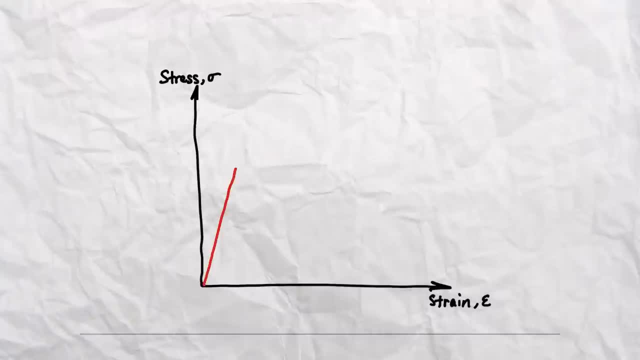 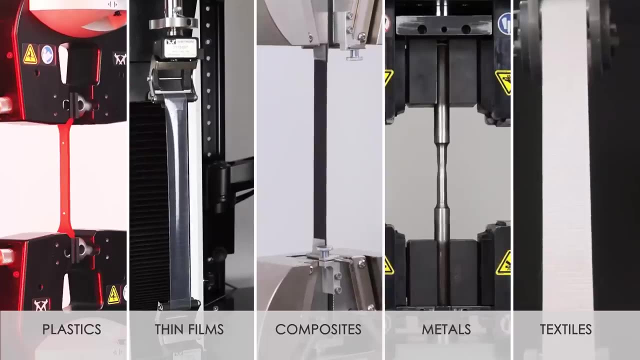 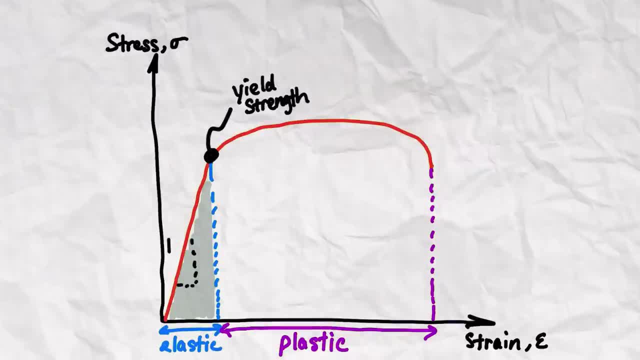 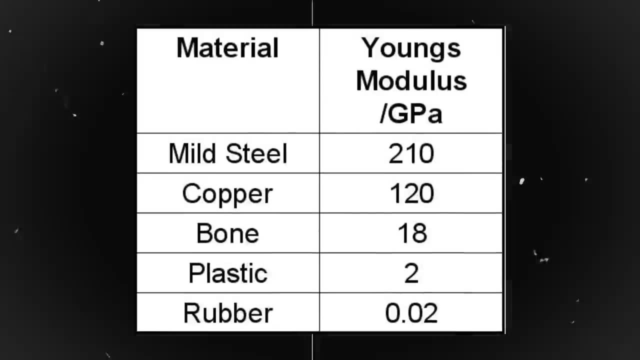 stay within this linear region. the slope of this line is a young's or elastic modulus represented by e and is the ratio of stress to strain within the elastic region. the higher the value, the more stiff a material is. any stress exceeding the yield strength will cause the material to permanently. 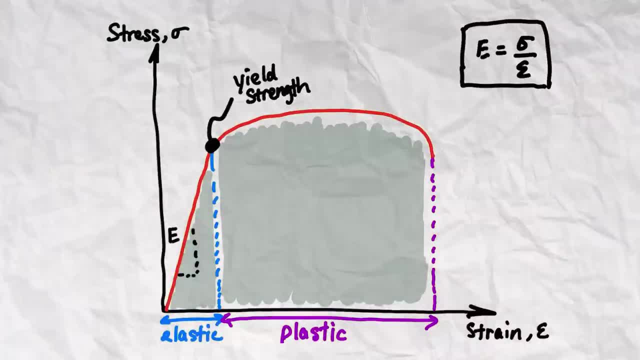 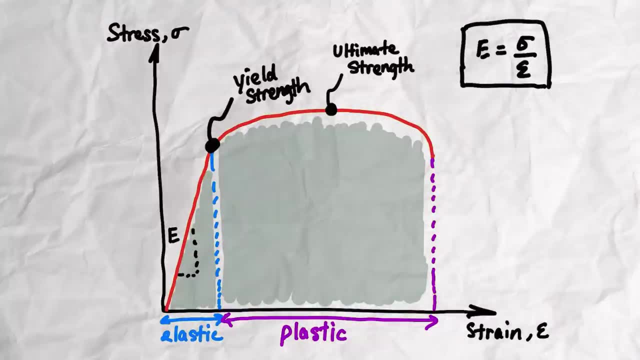 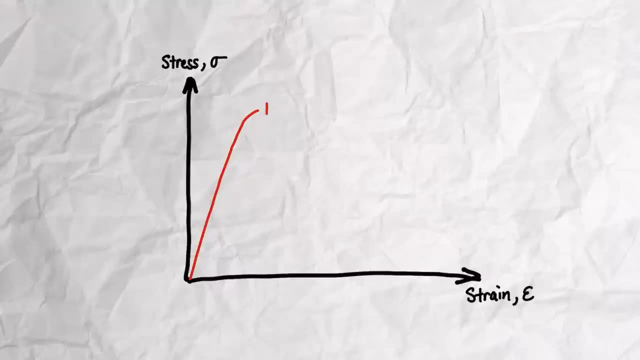 deform, which is this non-linear area known as the plastic region. the peak of this curve represents the ultimate strength of the material, which is the max stress a material can handle right before breaking. finally, this point is called the fracture point, which is the stress at which the material breaks. the stress drain curve for brittle materials will look something. 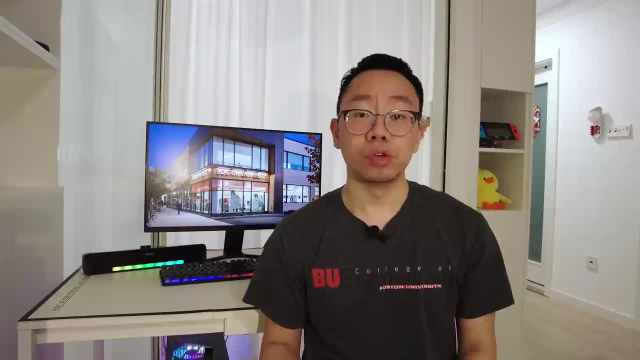 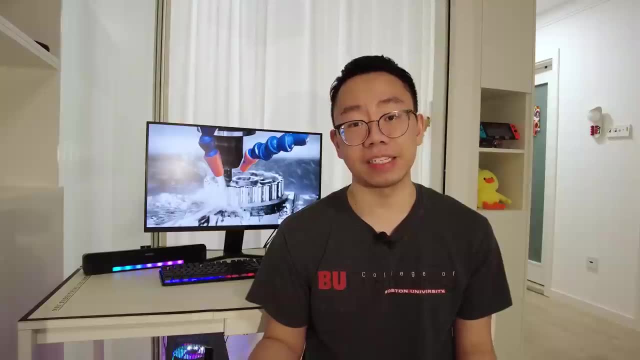 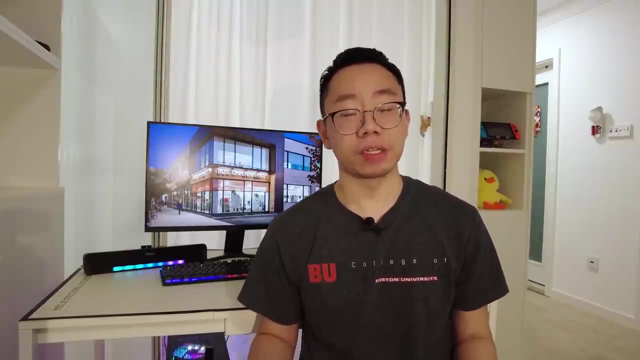 like this and for ductile materials it'll look something like this. you should be familiar with the stress drain curve and what the elastic modulus is for common engineering metals and steel, aluminum and polyethylene. now, a material can experience various forces and moments. the ones you should know include axial loading, which includes tension and compression, torsion and 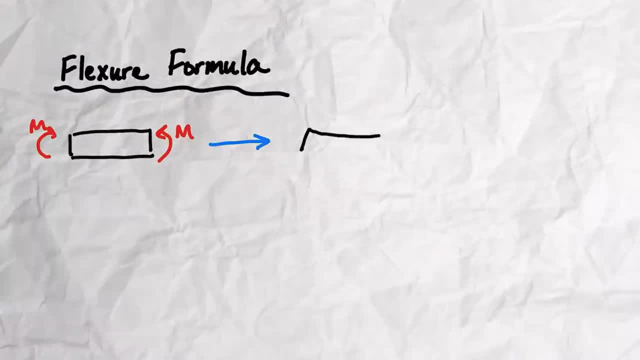 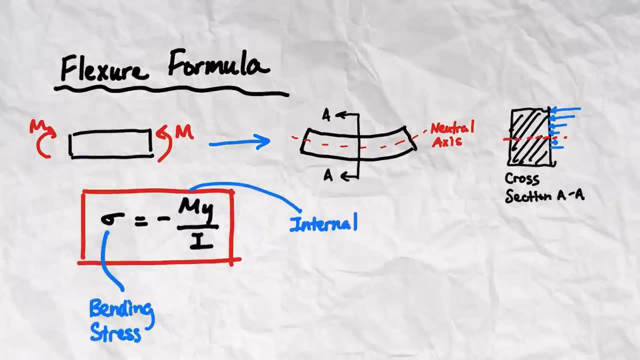 bending. when a beam is bent, you will use a flexure formula to calculate bending stress acting on it. sigma equals negative, my over i. sigma is the bending stress represented by these blue arrows. m is the internal bending moment, y is the distance from the neutral axis and i is the moment of. 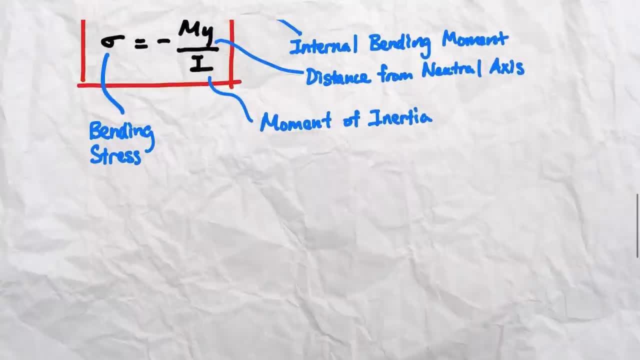 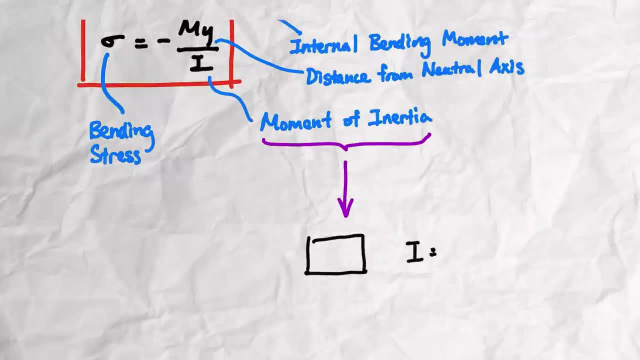 inertia. the moment of inertia will depend on your cross-section, geometry and location of the neutral axis. in this case it's a rectangle with the neutral axis passing through the centroid. so we have: i equals bh cubed over 12.. b is the width and h is the height, aside from the flexure formula. 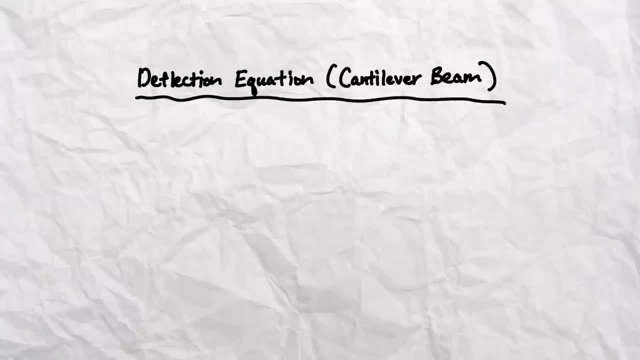 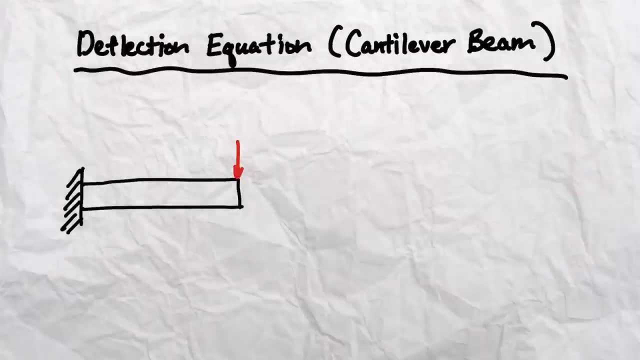 you should also know the deflection equation for a cantilever beam, which is a beam that has one fixed end and one free end, like this. to calculate the deflection when a force is applied at the free end, you can use this equation: delta equals f, l cubed over the center of the beam. 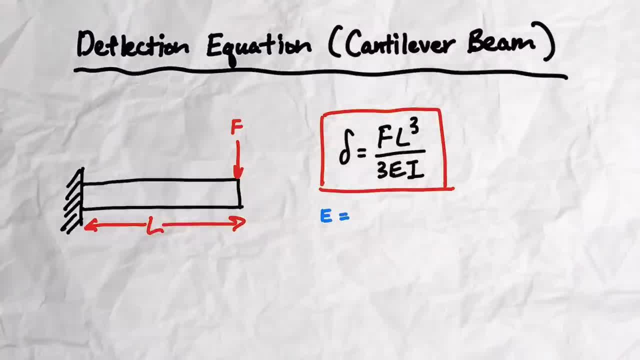 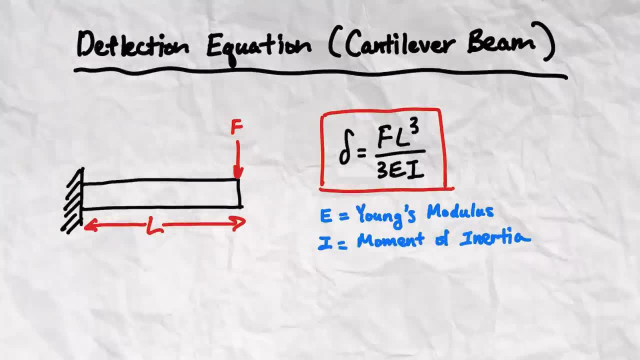 or three: e, i, f is the applied force, l is the beam length, e is the yon's or elastic modulus that we saw earlier in the stress strain curve, and i is the moment of inertia that we saw in the flexure formula. this deflection equation is specific for this beam configuration and will be different if. 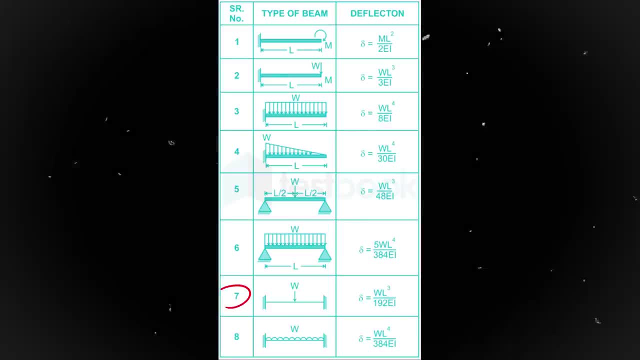 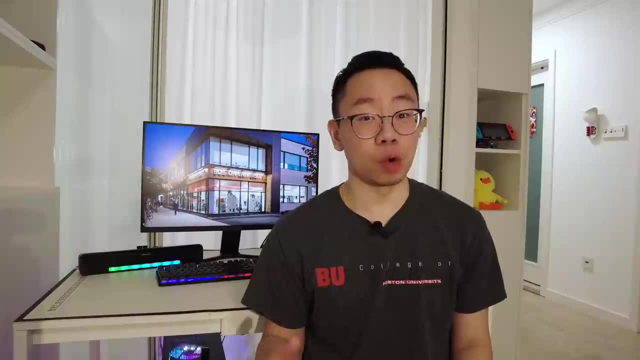 the location of the applied force changes, or say the beam is fixed on both ends. for some reason, engineers have this weird fascination with beams, so expect to get asked about this equation in a job interview. you should know how to calculate the maximum and minimum deflection and stress. 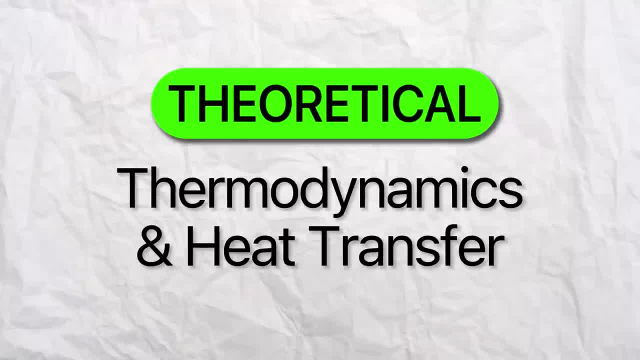 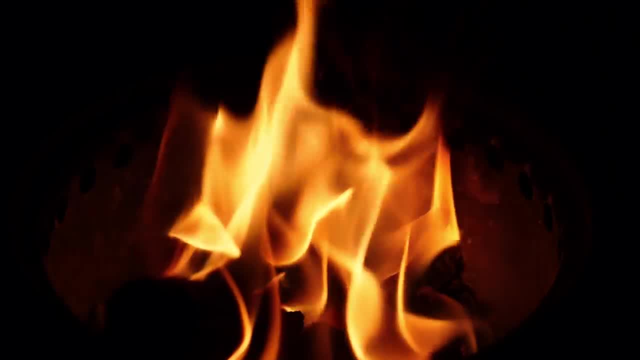 and where, along the beam, they occur. Next is thermodynamics and heat transfer. These were separated into two courses at my school and they're both equally important. While thermodynamics is a broad branch of physics dealing with the behavior of energy and matter in physical systems, 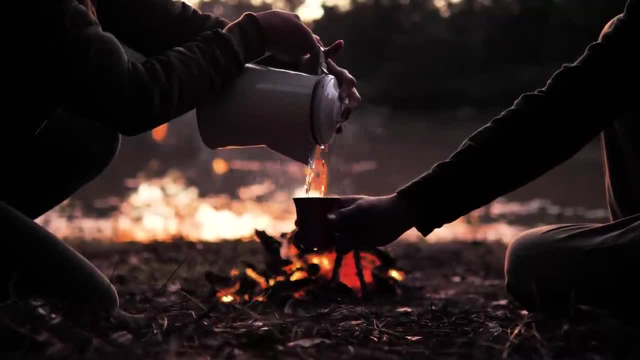 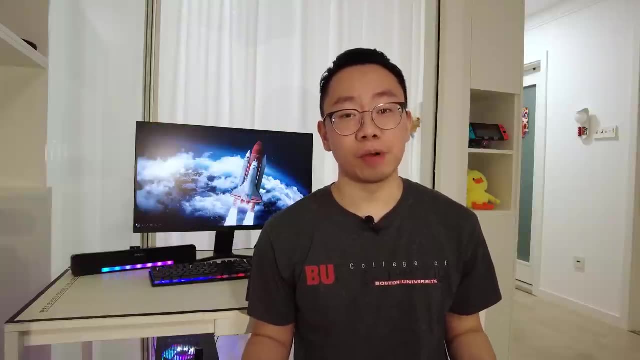 such as a rocket or refrigerator. heat transfer deals with the mechanisms and rates at which thermal energy is transferred from one object to another. There is a lot to know about thermodynamics, but for now start off by understanding the four laws of thermodynamics. 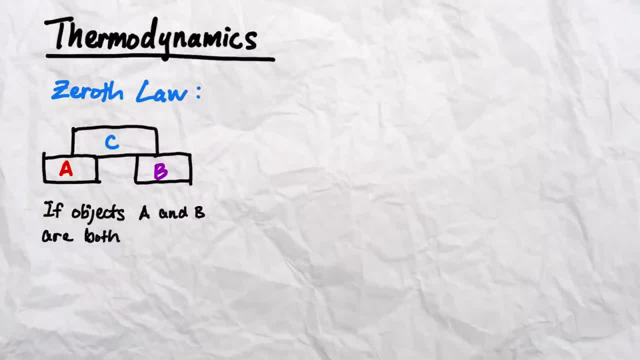 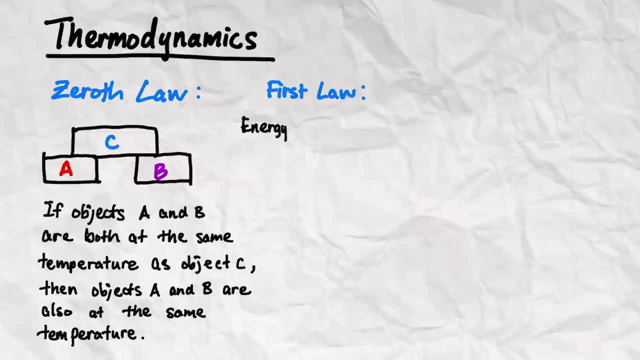 The zeroth law states that if objects A and B are both at the same temperature as object C, then object A and object B are also at the same temperature with each other. The first law says that energy cannot be created or destroyed in an isolated system. 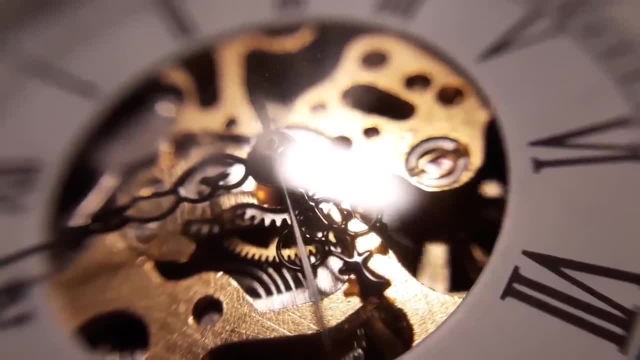 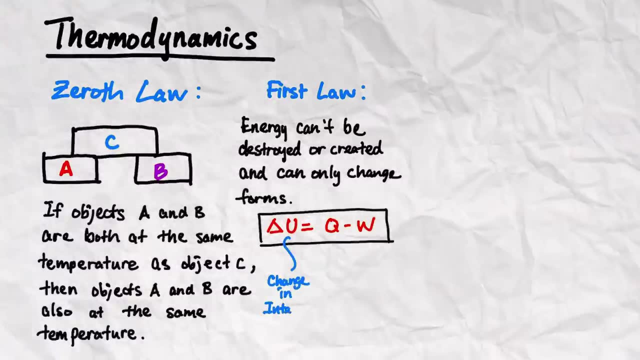 It can only change forms. In other words, the total energy within a closed system remains constant. The first law can be represented by: delta U equals Q minus W, Where delta U is a change in internal energy, Q is a heat added to the system. 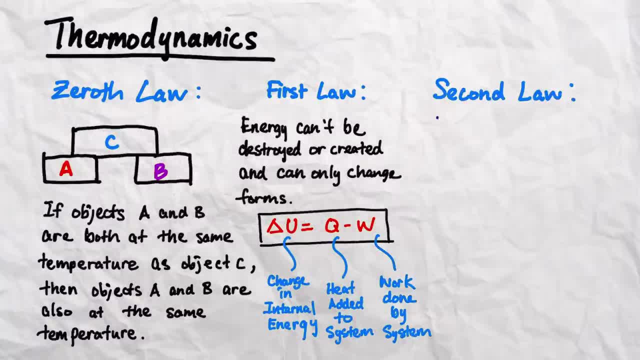 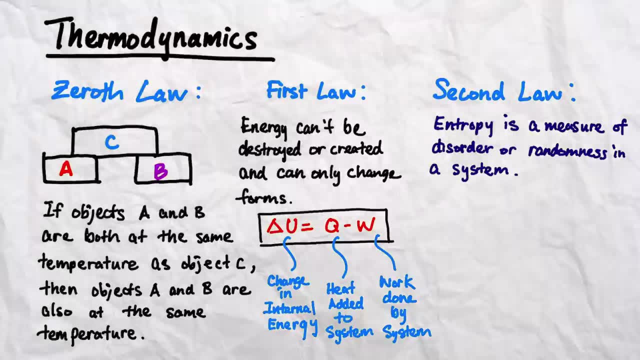 and W is a work done by the system. The second law of thermodynamics introduces the concept of entropy, which is a measure of the disorder or randomness in a system, and says three things. The first is heat flows from a hotter to colder object. 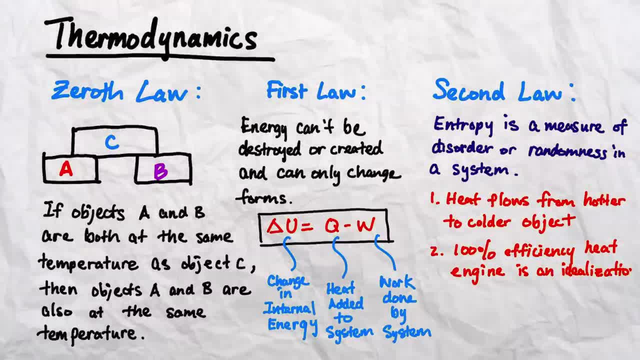 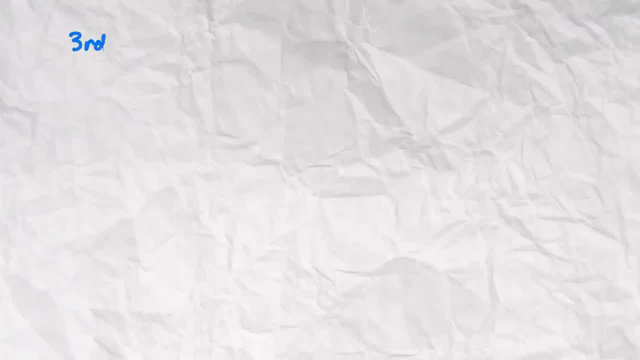 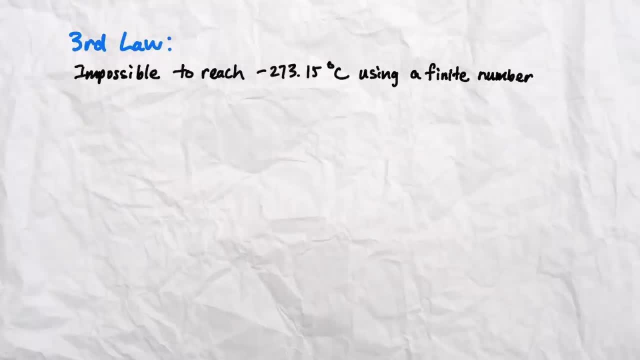 The second is it's impossible to create a heat engine with 100% efficiency. And the third is the total entropy of an isolated system always increases over time. Finally, the third law states that it's impossible to reach absolute zero or negative 273.15 degrees Celsius. 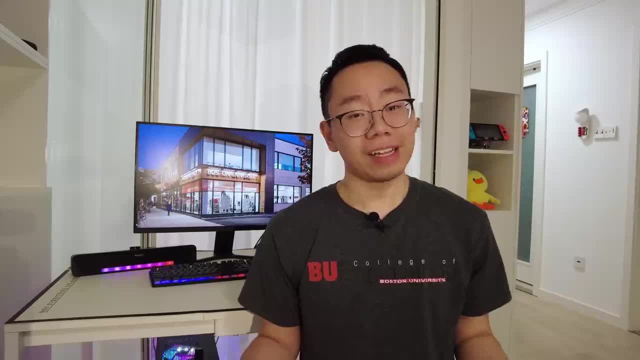 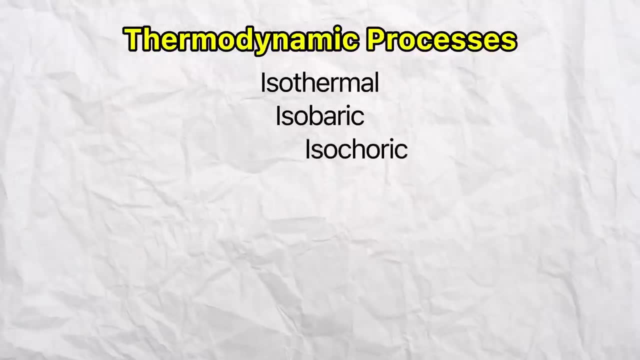 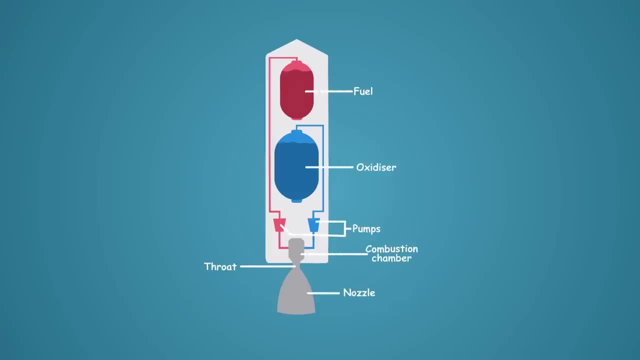 using a finite number of steps or processes. Finally, you should understand the different thermodynamic processes and their applications, like isothermal, isobaric, isochoric, isentropic and adiabatic. Take a rocket, for example. Fuel and oxidizer are mixed and burned. 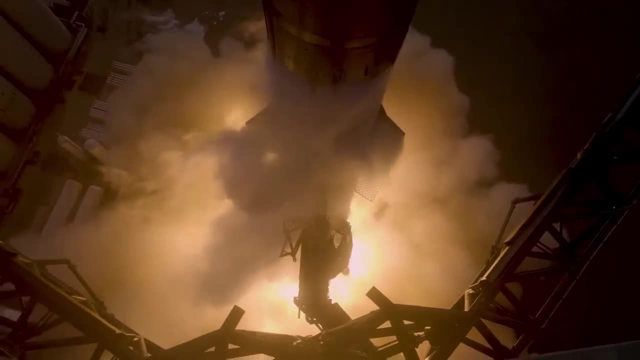 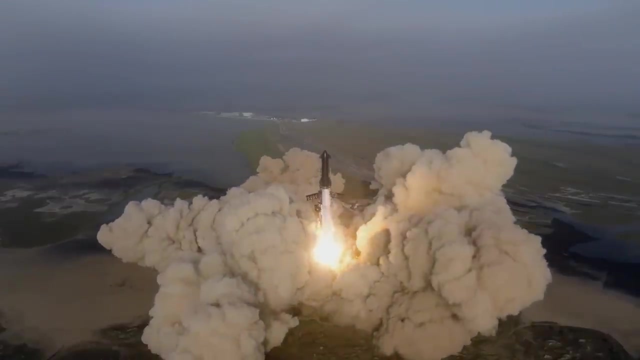 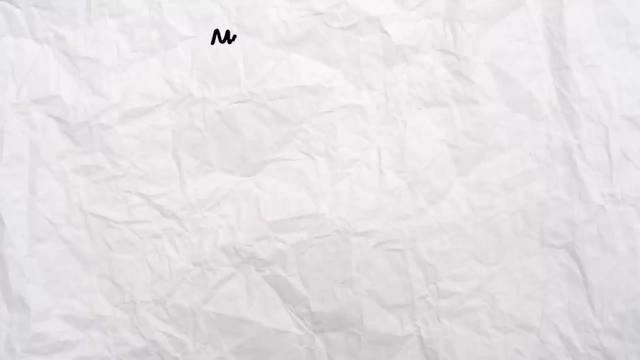 which results in higher temperature and pressure gases in the chamber. In other words, the gases expand as they pass through the rocket nozzle to generate thrust should be adiabatic For heat transfer. there are a lot of equations, but don't worry too much and start off by understanding. 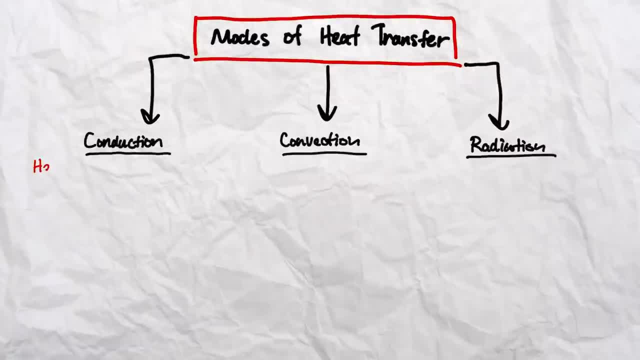 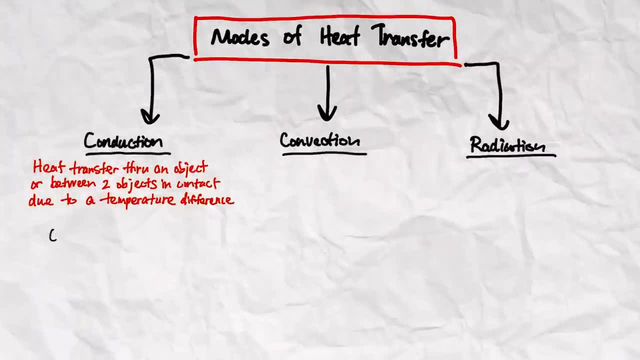 The three modes of heat transfer: conduction, convection and radiation. Conduction is when heat is transferred in an object or between two objects in contact due to a temperature difference and is represented by Fourier's law. Q dot represents the heat transfer rate. 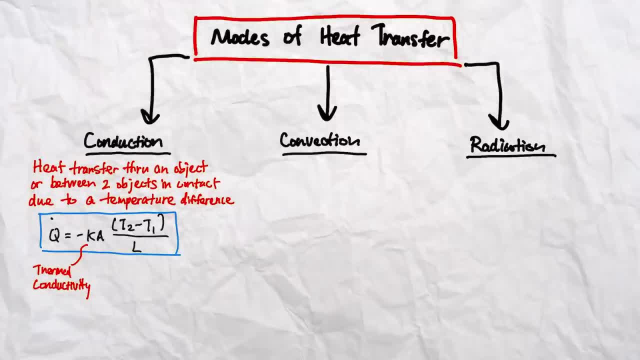 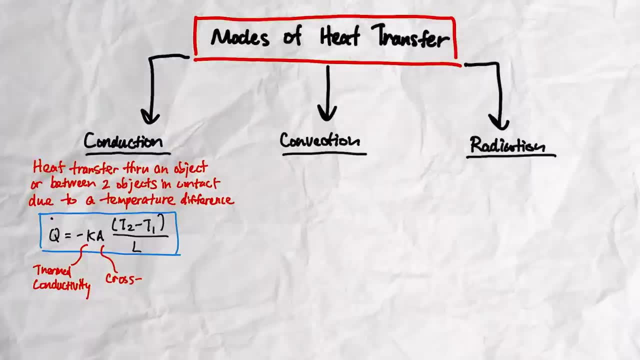 K is a thermal conductivity, which is a material's ability to conduct heat. For example, the thermal conductivity is excellent for copper and not so much for wood. A is the object's cross-sectional area, T1 is the temperature of the hotter end. 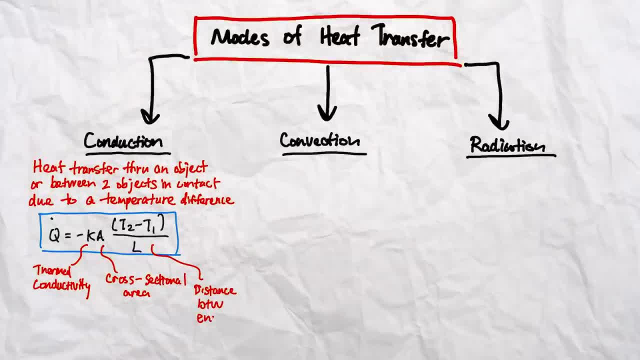 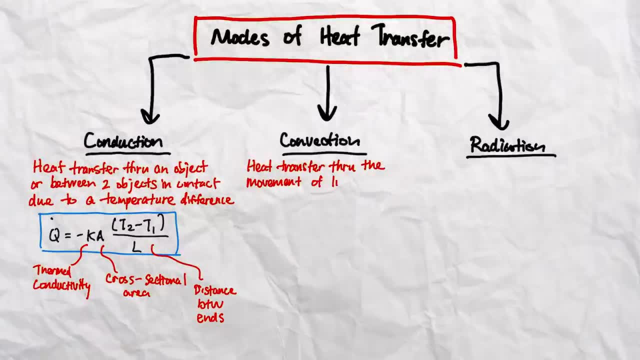 and T2 is the temperature of the colder end and L is a distance between them. Heating up a pan is an example of conduction. Convection is when heat is transferred by the movement of a liquid or gas and can be represented by Newton's law of cooling. 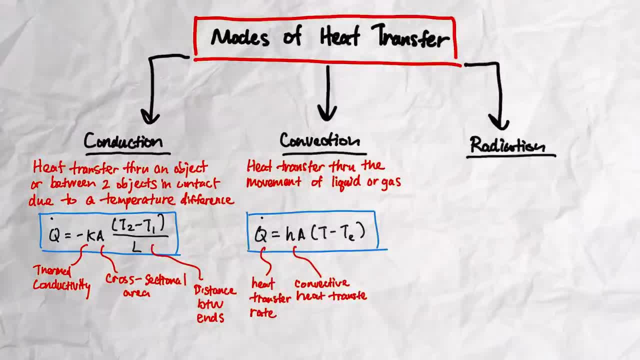 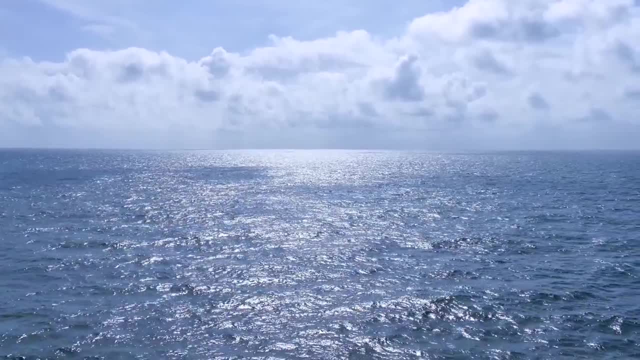 Q. dot is the heat transfer rate. H represents the convective heat transfer coefficient. The heat transfer coefficient is a fluid's ability to transfer heat. Water, for instance, is better than air at transferring heat. A is the surface area, T is the temperature of the object's surface. 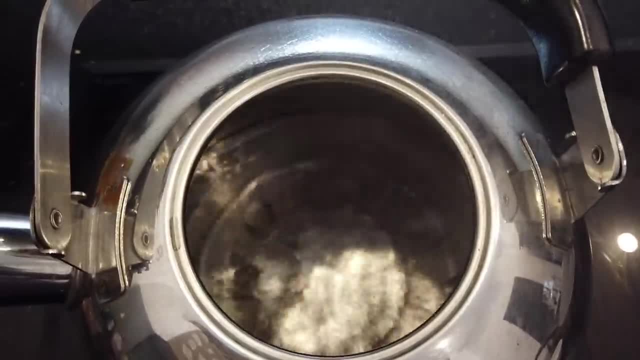 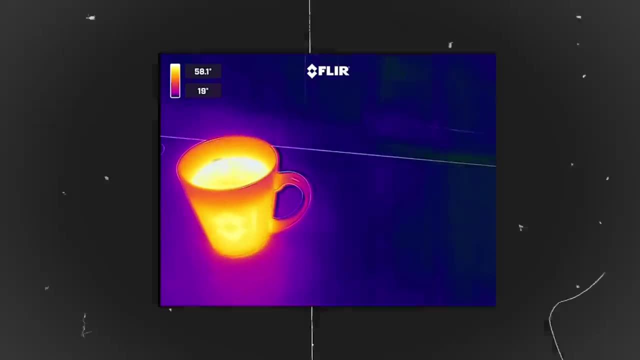 and Te is the temperature of the environment. An example is water boiling. Finally, radiation is when heat is transferred in the form of electromagnetic waves. All objects that you see emit thermal radiation. even if it doesn't feel warm, It can be represented by the Stefan-Boltzmann law. 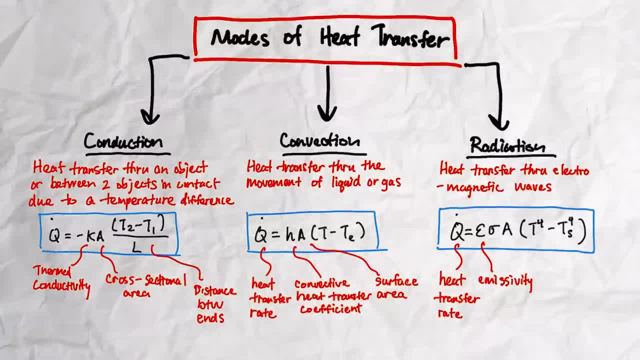 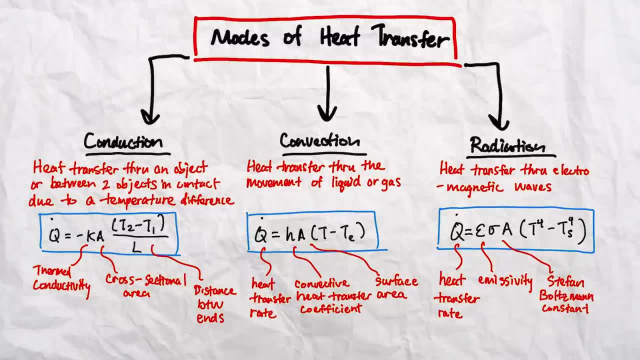 where Q, dot is a heat transfer rate. Absolutely, Epsilon is emissivity, which quantifies how effectively an object emits thermal radiation. Sigma is a Stefan-Boltzmann constant, T is the temperature of the radiating surface and Ts is a surrounding temperature. 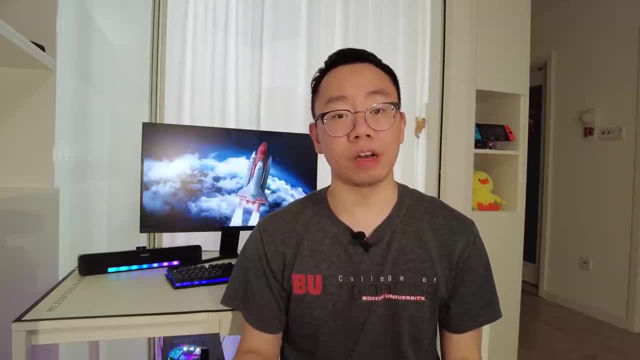 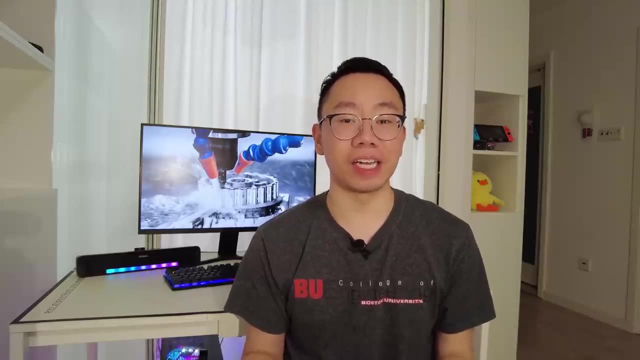 An example is the sun heating up the earth or warming yourself up with an electric heater. Now let's talk a little bit about fluid mechanics. Now I can sit here and talk about the concepts and equations from this class all day, But if I did that, this video will be several hours long. 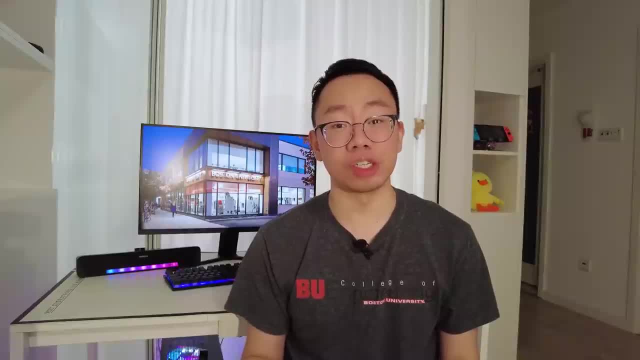 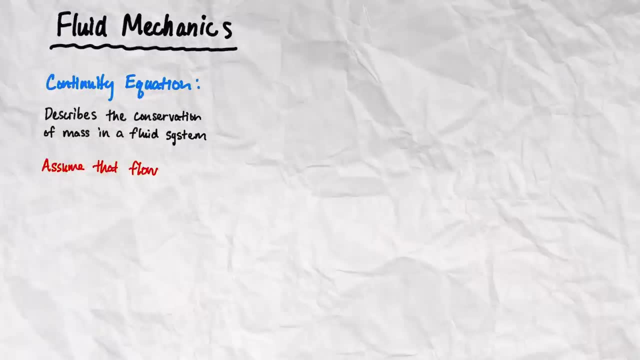 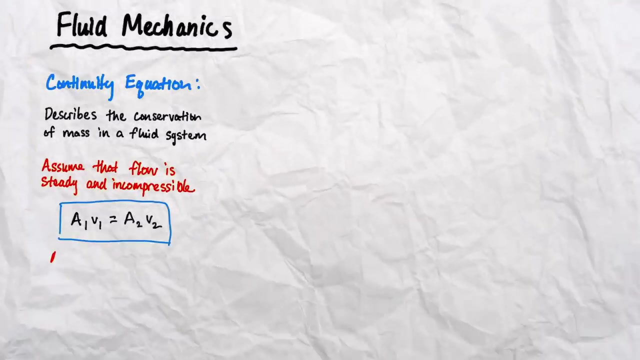 So I'll briefly mention three important concepts that you should definitely know. First is the continuity equation that describes the conservation of mass within a fluid system, Assuming the flow is steady and incompressible. it can be represented by A1 times V1 equals A2 times V2.. 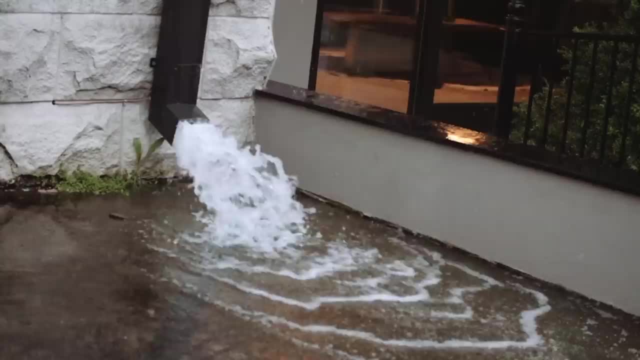 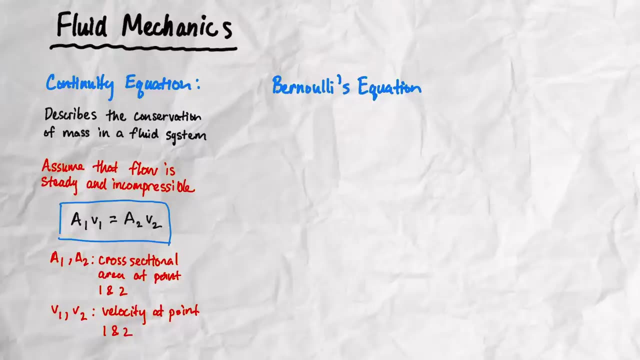 A1 and A2 are the cross-sectional areas at point one and two. in say a pipe or tube, V1 and V2 are the velocities at points one and two. Second, you should know about Bernoulli's equation that describes the conservation of energy. 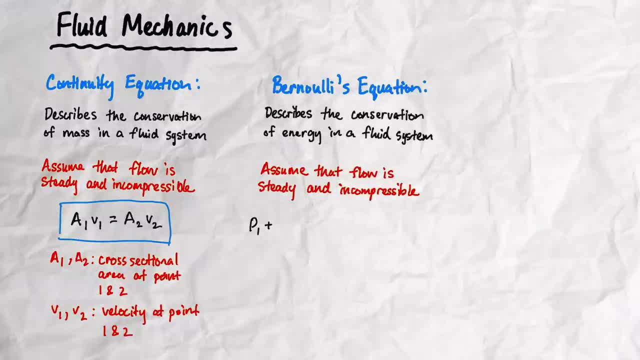 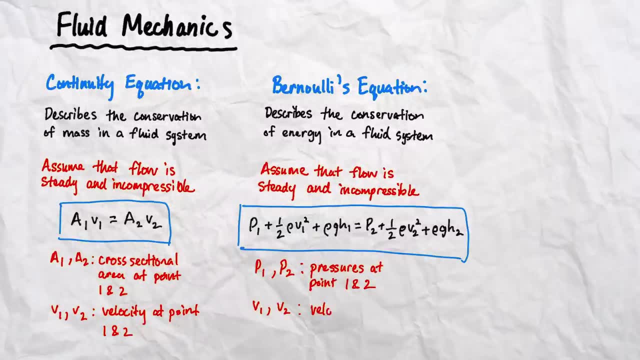 for a fluid, Assuming that the flow is steady and incompressible, we can apply the equation to a single streamline in a fluid where P1 and P2 are pressures at points one and two. V1 and V2 are velocities at points one and two. 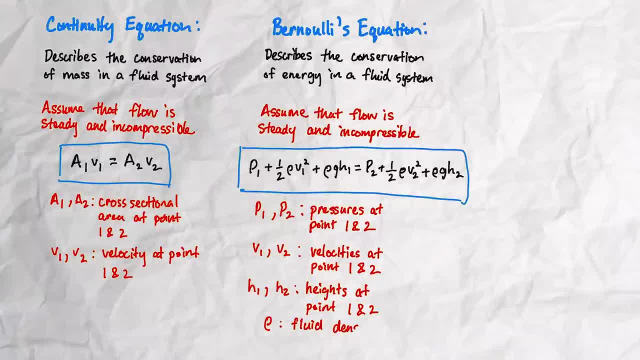 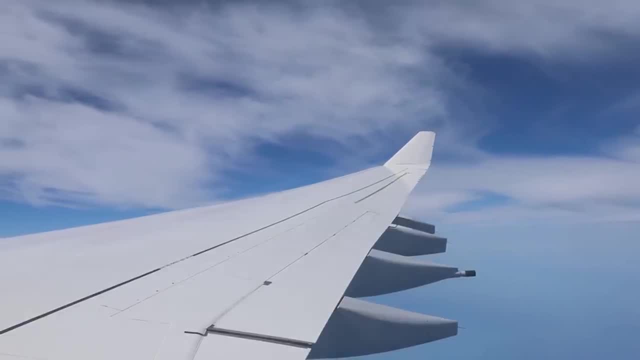 and H is the height at points one and two. Rho is the fluid density and G is a gravitational acceleration. This equation can be used to analyze flow across an aircraft wing. Finally, we have the Navier-Stokes equation, which is a set of partial differential equations. 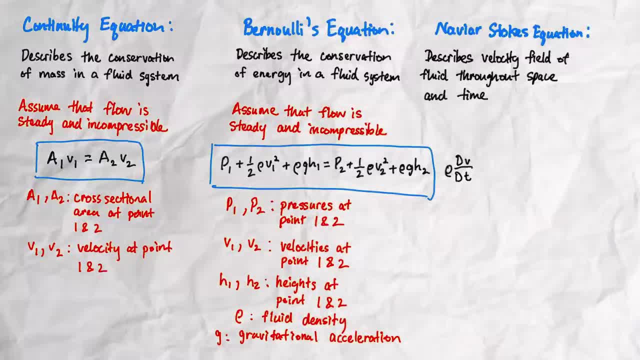 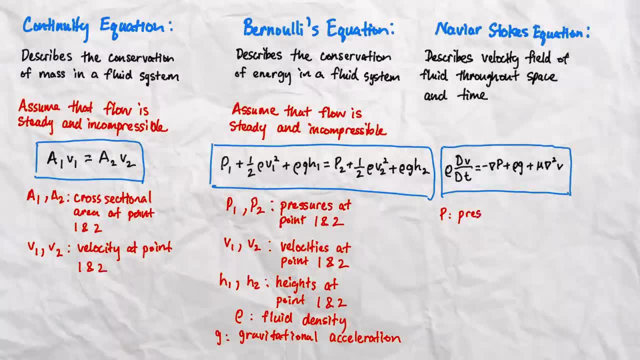 used to describe the velocity and a fluid throughout space and time and accounts for effects of pressure gradients, viscous forces and gravitational forces. P is a pressure, V is a velocity, mu is a dynamic viscosity. rho is the fluid density. 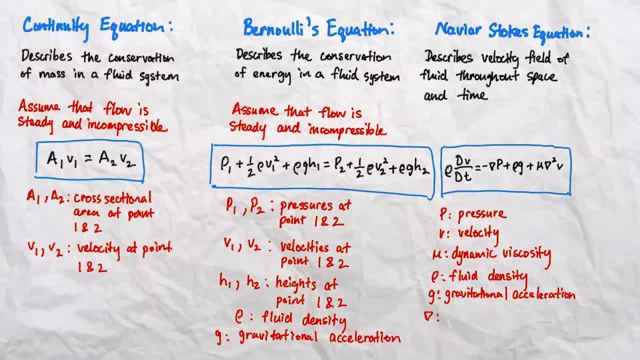 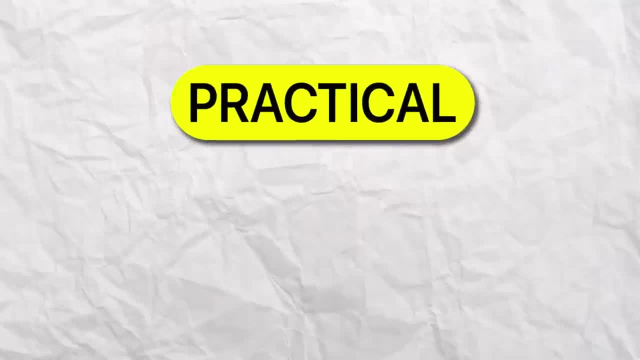 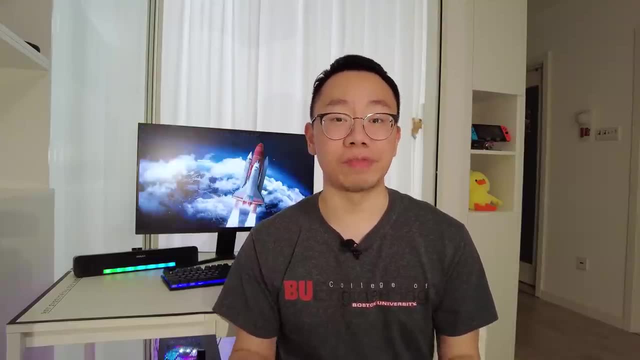 G is a gravitational acceleration and inverted delta represents divergence, which just takes a vector field to produce a scalar quantity such as pressure or velocity. Moving on to the more practical classes, we have manufacturing processes. This class is very important because you learn about how different parts are created. 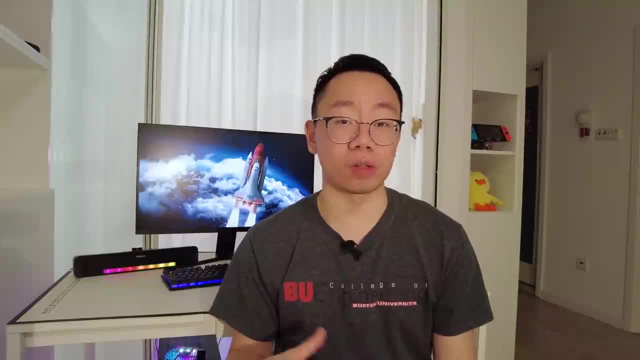 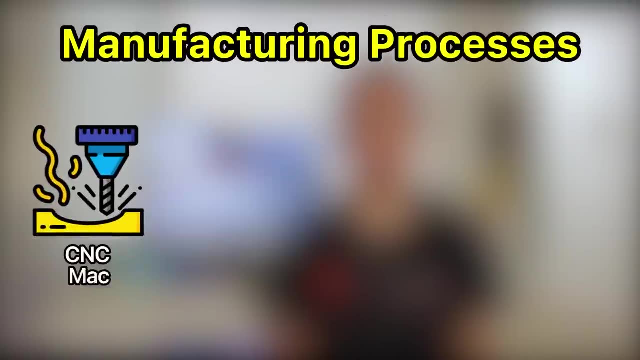 using a variety of manufacturing methods based on the part, design part, material, annual volumes, costs and lead times. The most popular one that engineers use are CNC machining, injection, molding, sheet metal forming and 3D printing. CNC machining is a subtractive process. 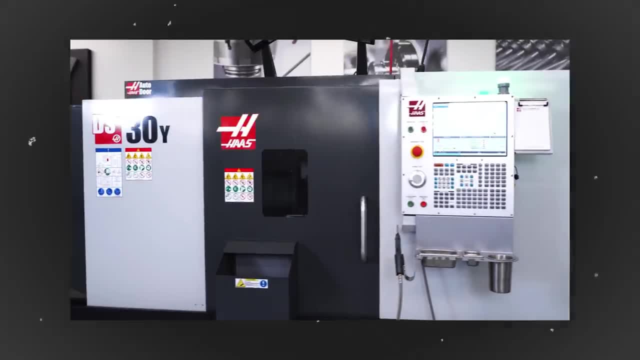 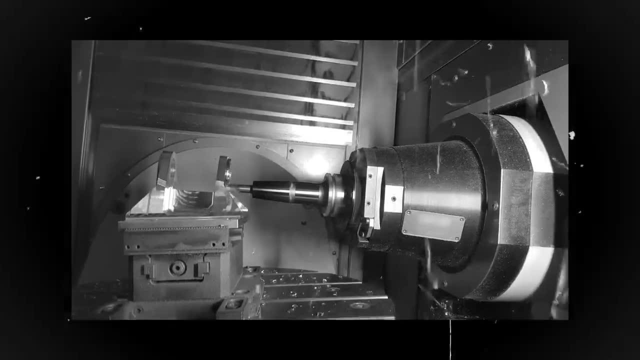 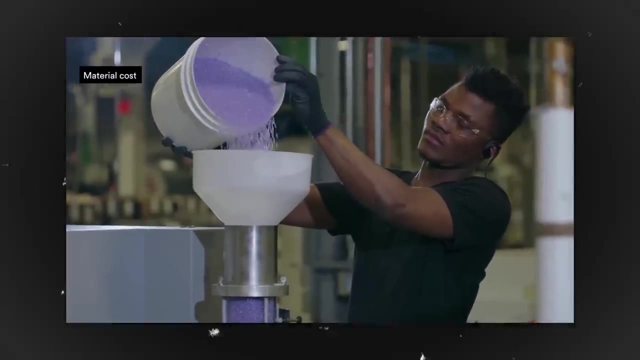 that leverages milling machines and lathes programmed with G-code to generate tool paths and precisely remove material from a piece of plastic or metal raw material to create complex features and shapes. Injection molding is great for high volume applications. that takes plastic pellets and loads them into a hopper. 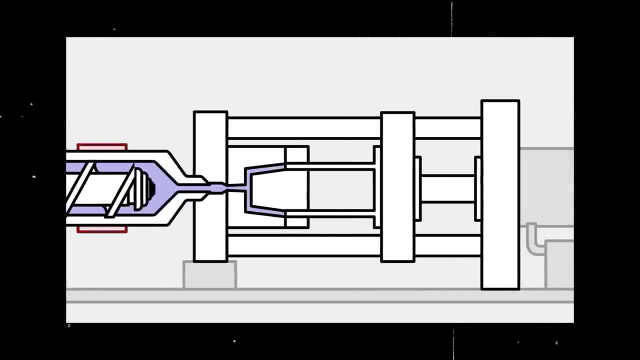 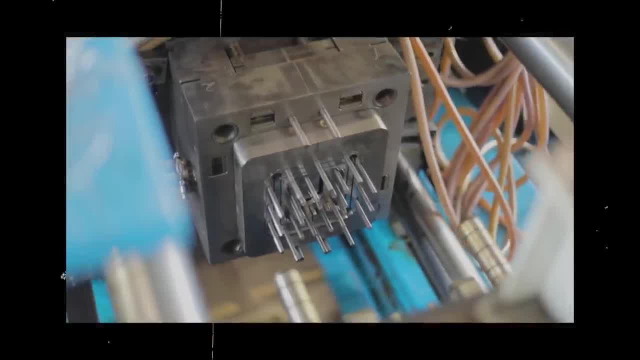 As the plastic pellets are pushed forward by an auger, they melt and the molten plastic fills a mold cavity where it cools, solidifies and is ejected from the mold core by ejector pins. The part is finished and the process repeats all over again. 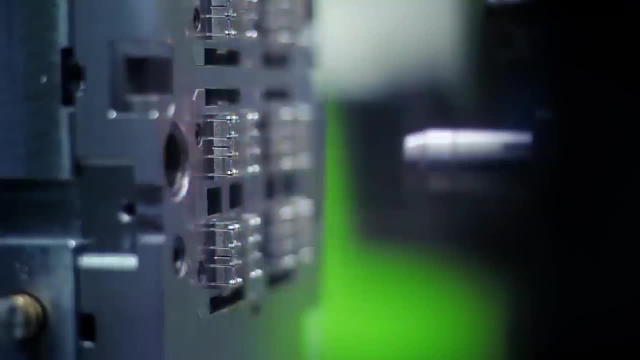 Without injection molding we would never come to know the wonders of Legos. Sheet metal forming is when you get a mold, or the roughness of the mold and the thickness of the mold. Sheet metal forming is when you take a flat sheet of metal. 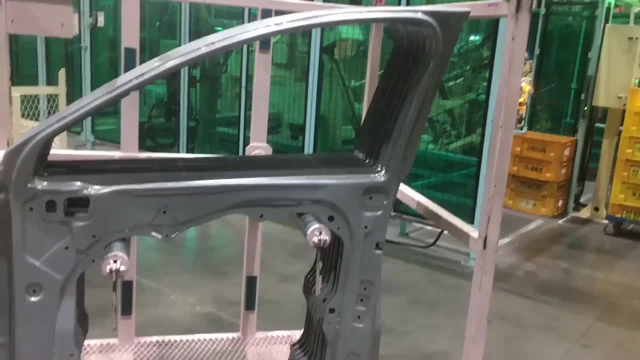 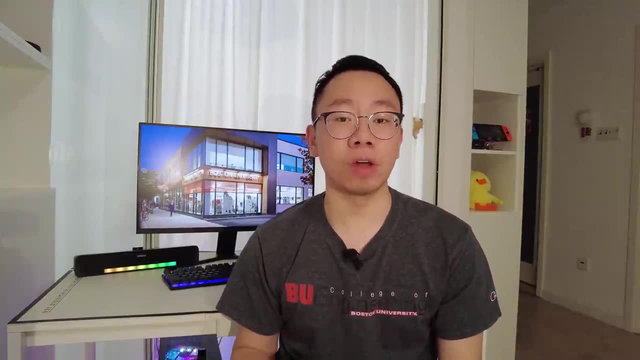 deform it by applying a force, using various methods such as bending, stretching and stamping. Car door panels, for instance, are made with this process. Engineers rely on 3D printing to make prototypes and even low volume end-use parts. 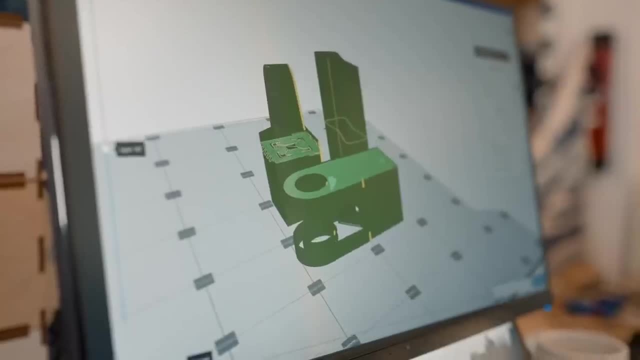 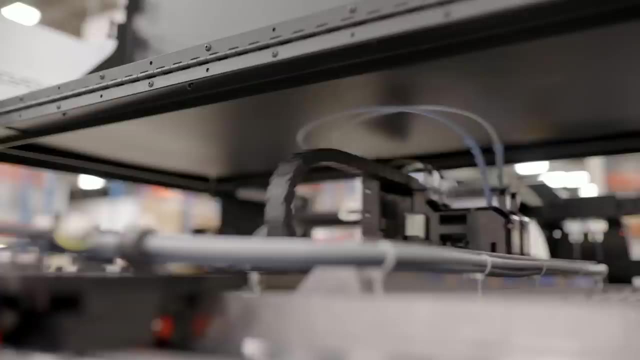 To 3D print a part. engineers will take their 3D CAD model and save it as an STL file where the 3D model is sliced into very thin horizontal layers. The printer adds one layer on top of another following the instructions from the slide guide. 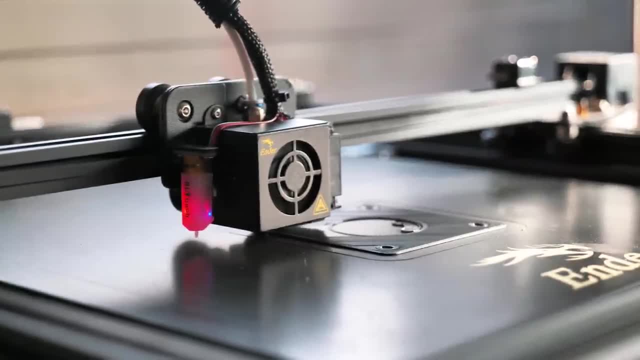 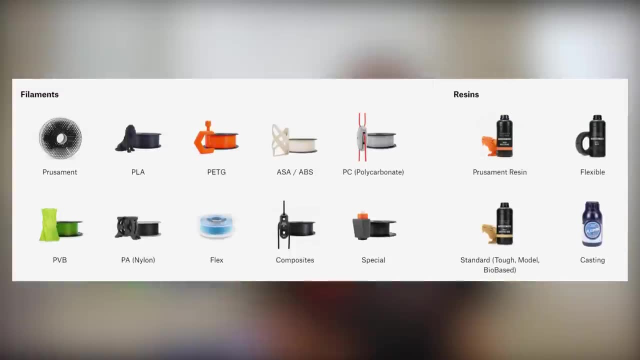 sliced file, and the material cools and solidifies after being extruded from the nozzle. Most 3D printers print in plastic, but there are also metal and ceramic ones. The material is usually in the form of a spool of filament or powder, depending on which technology the printer uses The most. 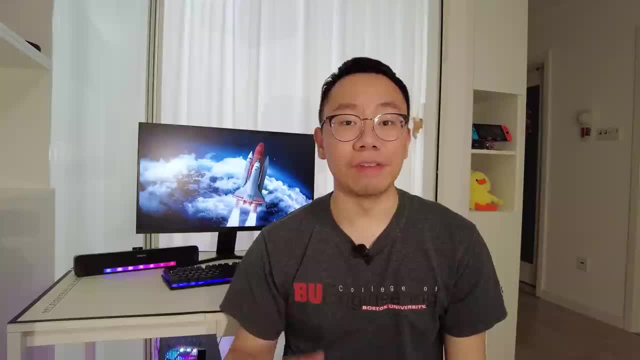 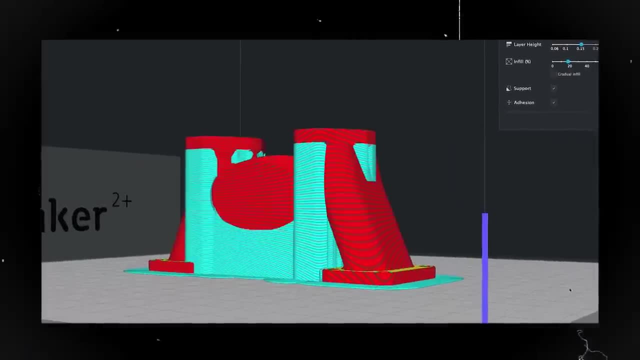 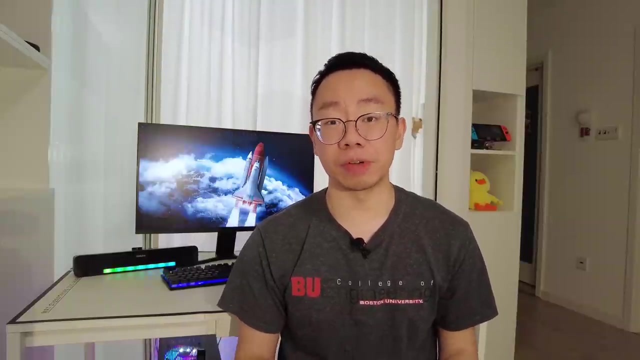 popular ones are FDM, SLA and SLS. If your part has complicated features like overhangs or undercuts, the printer will add temporary support structures like these that can be removed after the print. As an engineer, you should be well-versed in design for manufacturing or DFM principles. 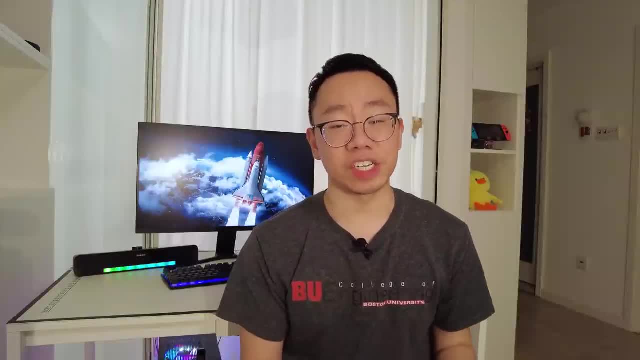 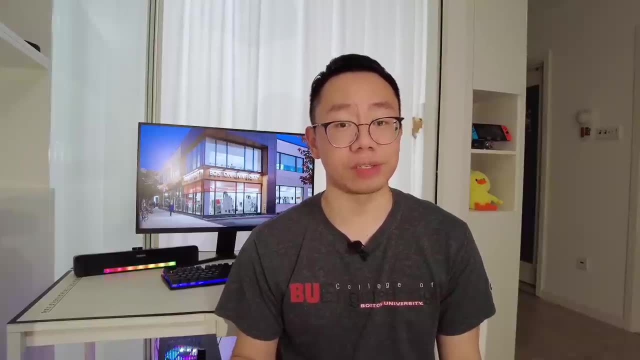 For example, if you're designing a CNC milled or plastic injection molded part, you will need to apply the rules of thumb and design guidelines for each particular manufacturing process. In a nutshell, a plastic injection molded part should consider things like uniform wall thickness. draft. 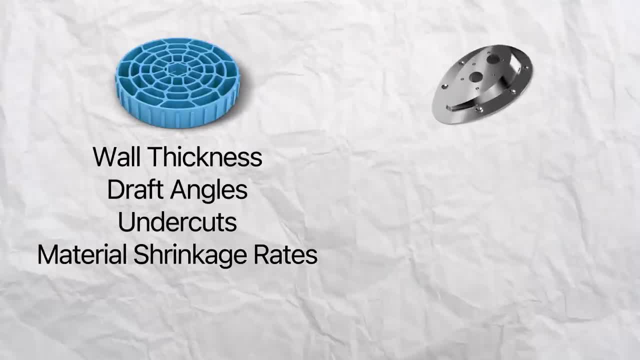 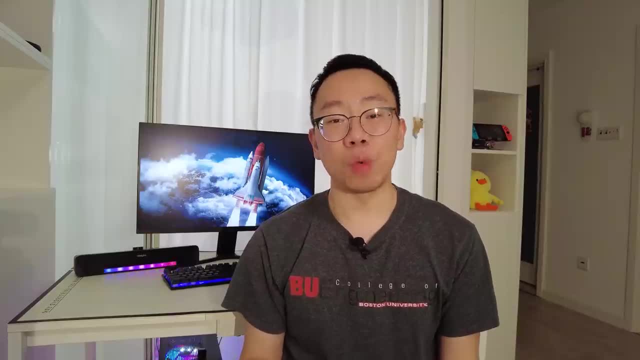 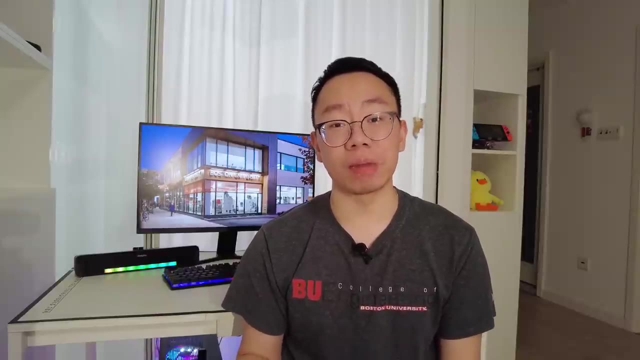 angles, undercuts and material shrinkage rates, While a CNC milled part should avoid deep, narrow features, sharp corners, custom molding holes, sizes and threads. If you look at any well-designed product- take this iPhone, for example- hundreds upon thousands of iterations and prototypes for each component were made and 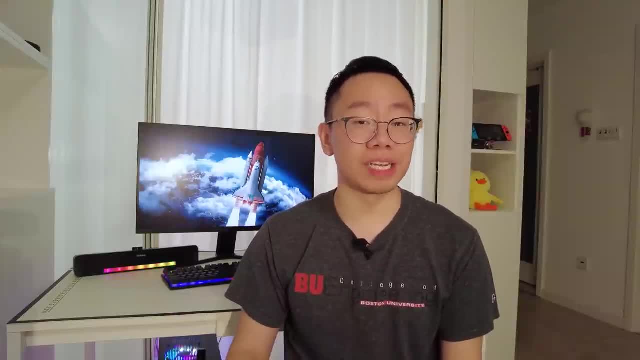 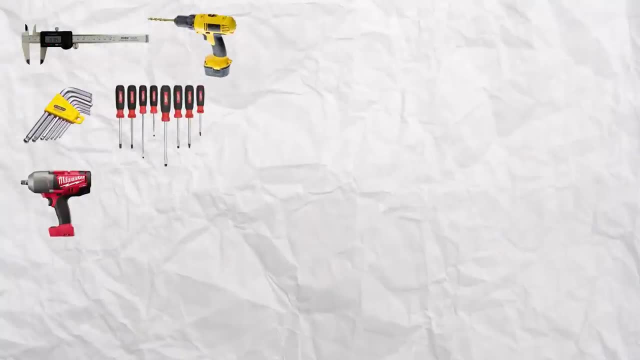 tested. To build these prototypes, you will need to know how to use some essential tools and machinery. Hand tools include calipers, hand drills, allen keys, screwdrivers, impact drivers and deburring tools. Equipment and machinery that are good to know include CNC machines, 3D printers. 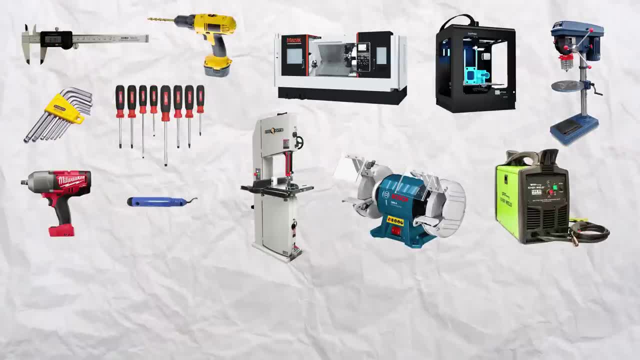 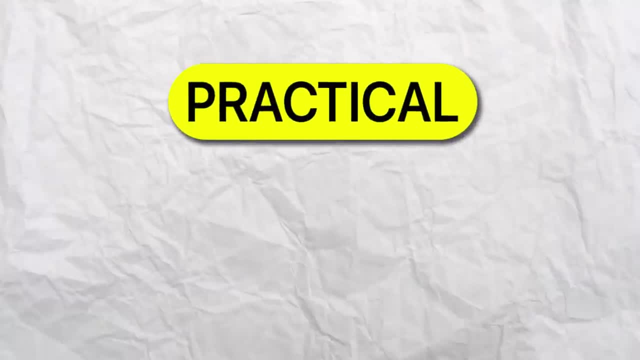 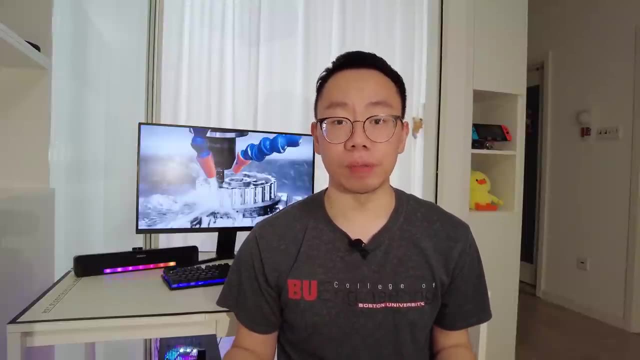 drill presses, bandsaw bench grinders, welding machines, sheet metal machines, injection molding machines, soldering irons, multimeters and oscilloscopes. Saving the best for last, we have Electromechanical Design class. This class equips you with practical skills that make you employable. First, you should become an 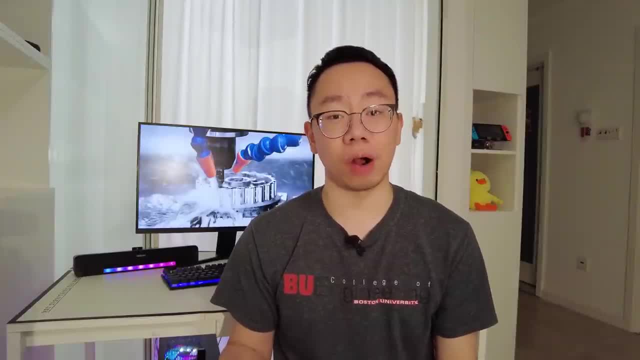 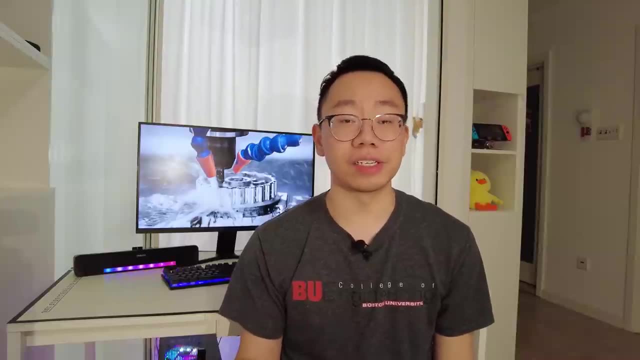 expert at using at least one CAD software to design parts, such as SolidWorks, Creo, CATIA, NX, Inventor or Solid Edge. Most of these offer student editions, so just pick one to learn and practice modeling anything you can find. There are plenty of tutorials on YouTube to help you get. 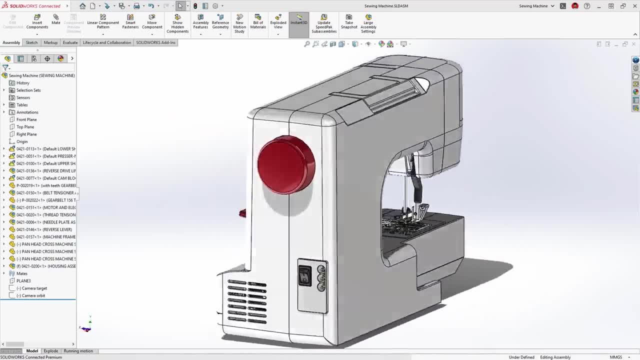 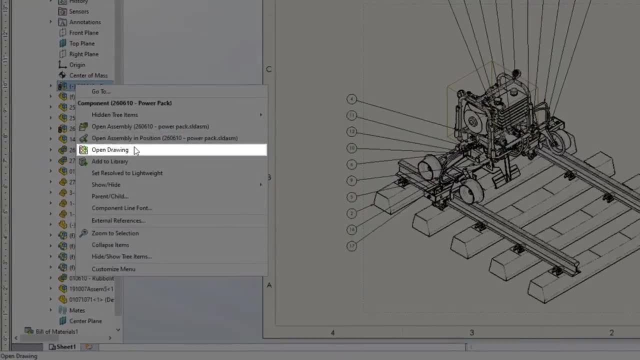 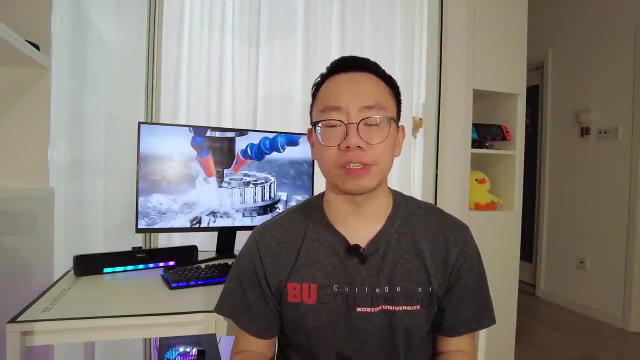 started. Mechanical engineers use CAD to design 3D parts and assemblies of actual products, as well as to make 2D technical drawings so that these parts can be manufactured according to engineering specifications. For every part you design in class or for a club, think what manufacturing process. 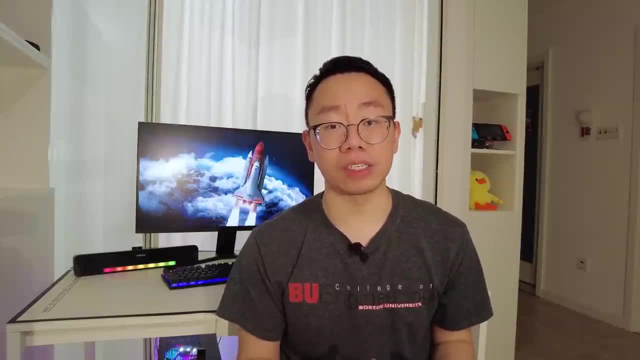 you would use to make it and how you can optimize part design to improve manufacturability and cycle time without sacrificing your time and effort. If you have any questions, feel free to ask them in the comments section below. If you have any questions, feel free to ask them in the comments section below. 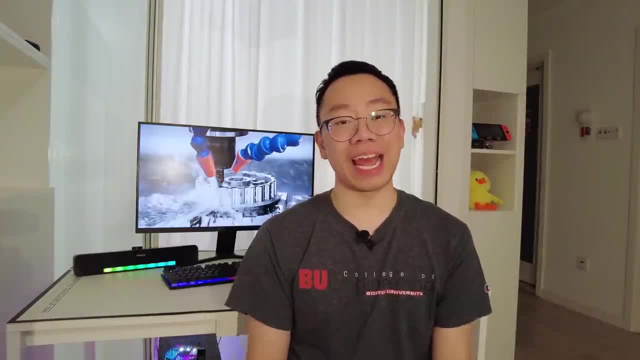 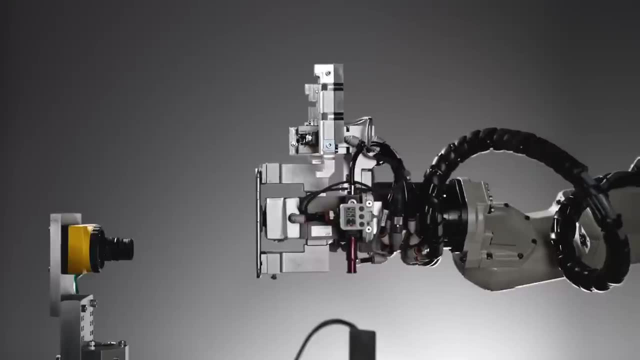 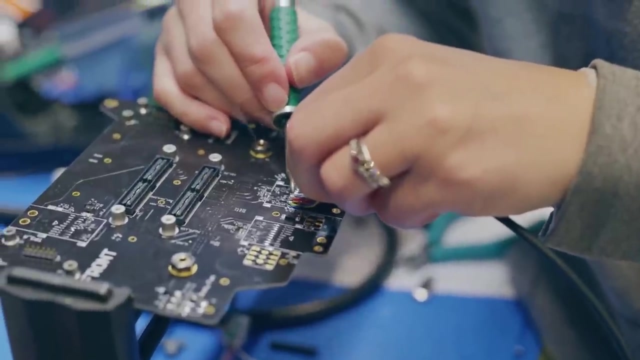 Now, even though we're mechanical engineers, virtually every product in the real world, such as iPhones, robots, aircraft and cars, involve moving parts and electronics, So another valuable skill that you should have is building simple circuits using breadboards and knowing how. 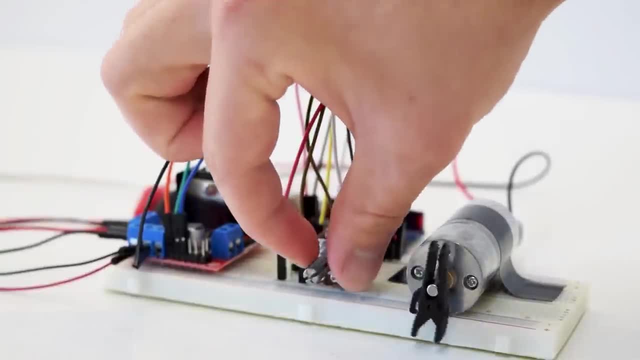 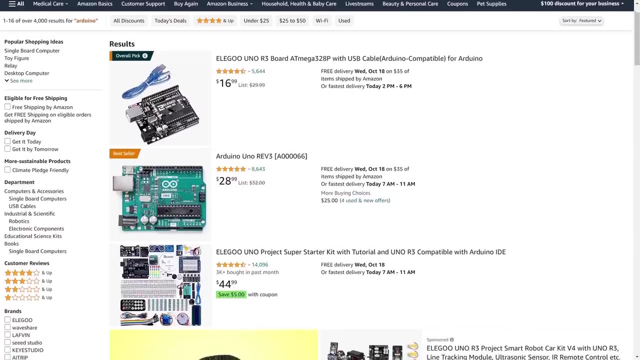 to program microcontrollers to control sensors, motors, valves and lights. Familiarize yourself with different types of brush and brushless motors, encoders and sensors. If you want to get started, I highly recommend you check out my video on how to build a mechanical engine using CAD software. 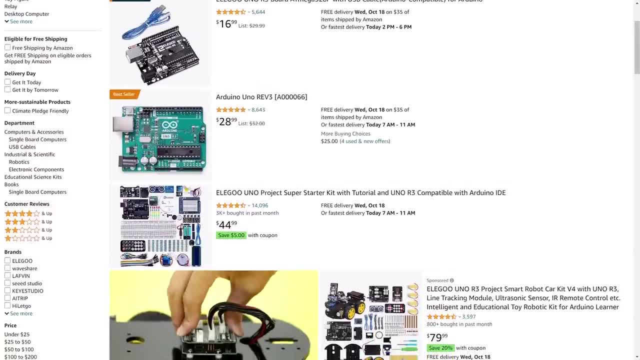 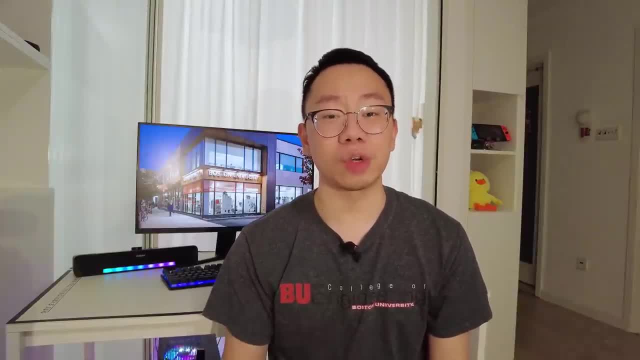 I highly recommend getting an Arduino or Raspberry Pi kit on Amazon Link in the description below if you're interested. Now, once you step foot in industry, you can't just go up to a machinist or your manufacturer and say, hey, here are the CAD models of all the parts I just designed Make. 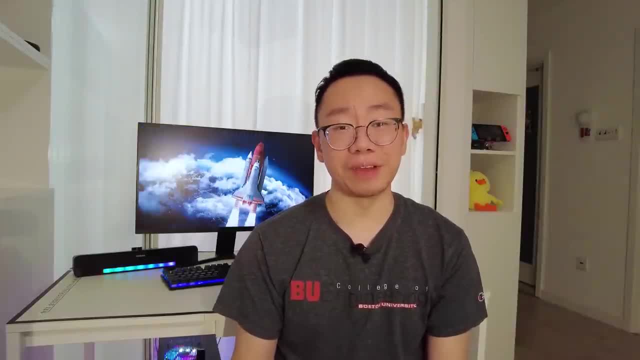 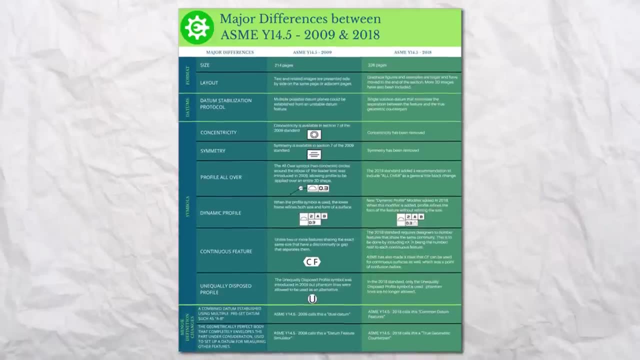 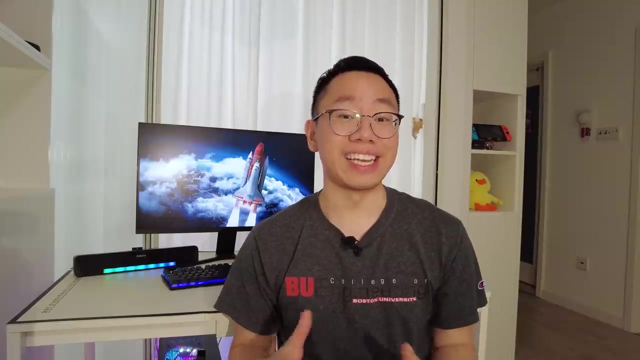 them. for me, They will basically wipe you off the face of this planet if you do that. So instead, as an engineer, you need to make professional 2D technical drawings that follow ASME Y14.5 GD&T standards. GD&T stands for geometric dimensioning and tolerancing, and it's the universal language. 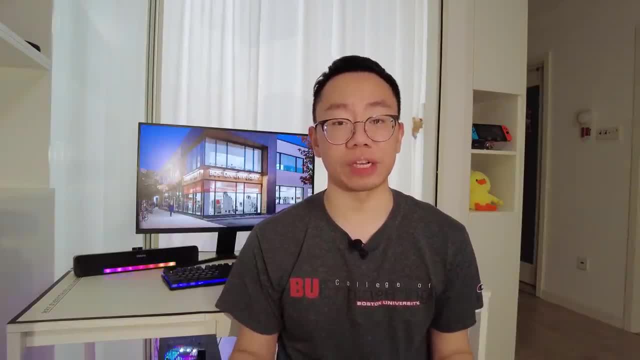 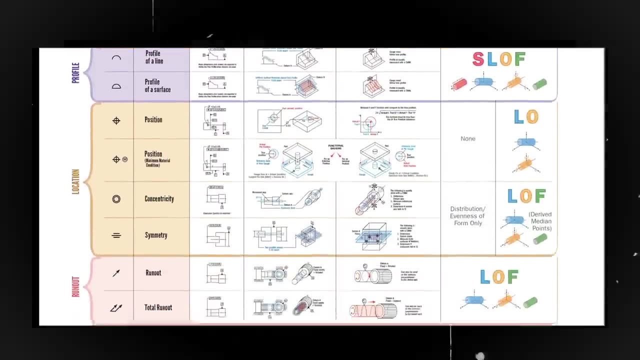 for communicating tolerances and geometries on a drawing. There are 14 symbols in total that describe how flat a part surface must be or where a slot or hole feature must be exactly located. You should know what all of these symbols represent and when to use datums. For example, if I called 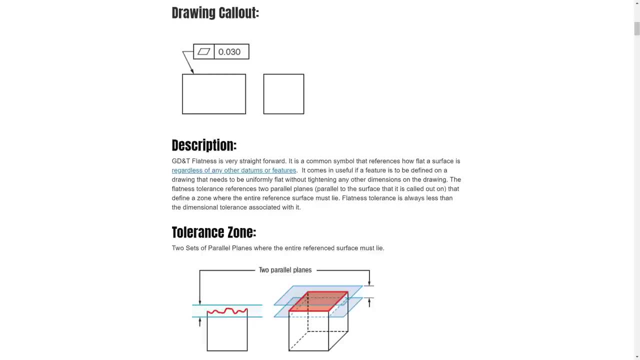 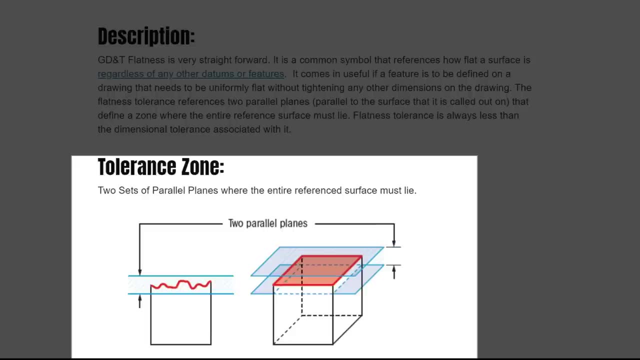 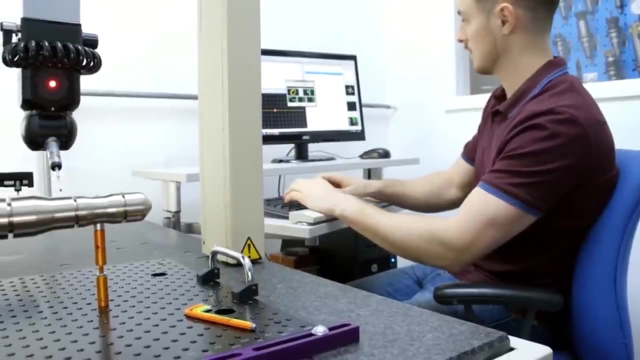 out this flatness symbol for a part surface. the final surface must fall between these two blue planes parallel to it, One that's 0.03 inches above and another one that's 0.03 inches below it. A quality engineer or a technician will use a CMM or OMM to check if the part meets this specification. 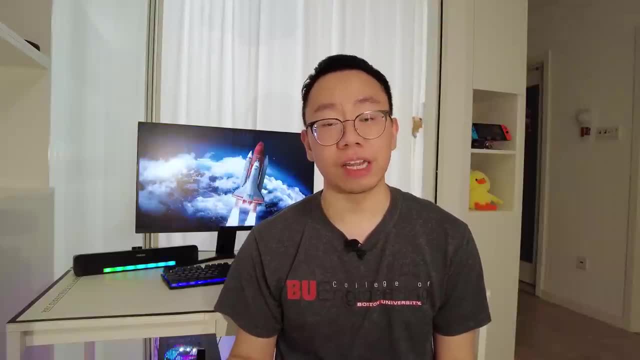 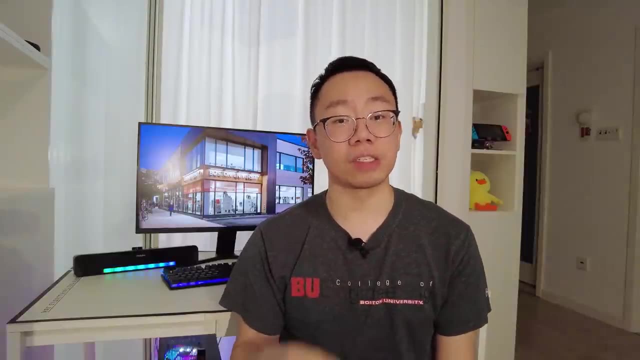 Now, before engineers send parts off to be produced, they first need to perform a tolerance stackup analysis to ensure all the parts will fit together seamlessly based on the tolerances called out on the drawing. Tolerance is the allowable amount of variation of each of the. 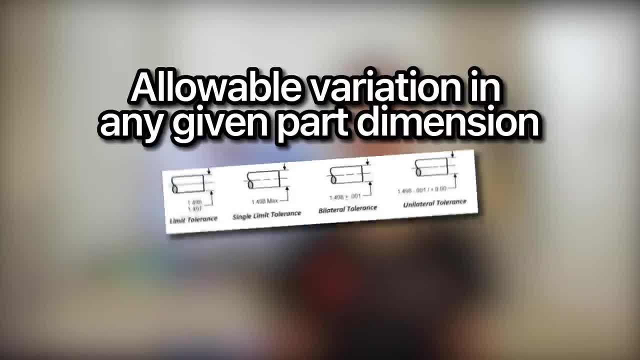 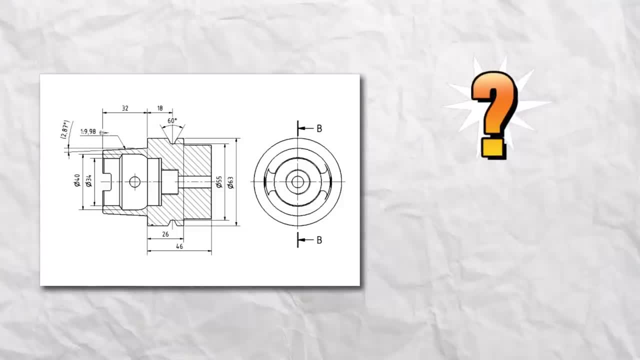 parts in any given part. dimension. Types of tolerances you can call out include limit, unilateral and bilateral, For every dimension on a drawing. ask yourself if it's critical and if you can get away with calling out a standard tolerance of 0.005 inch, or do you need a super tight? 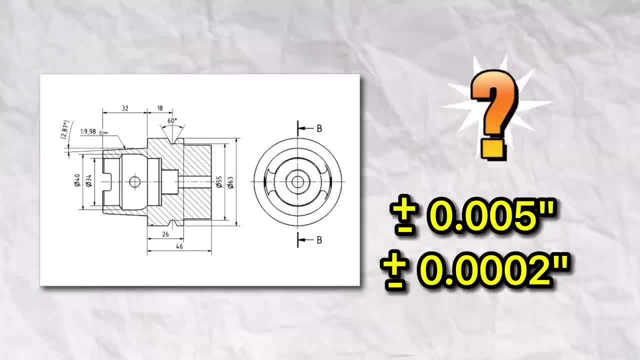 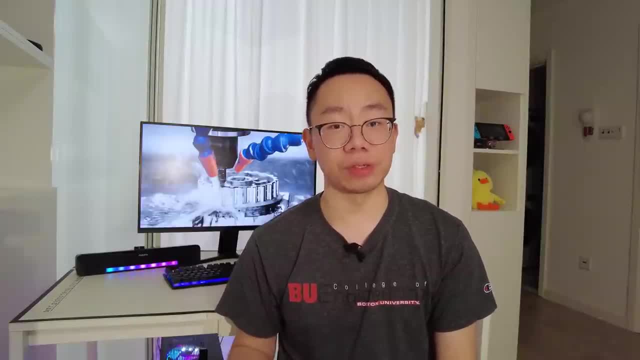 tolerance of 0.002 inch based on the part's function. Inexperienced engineers tend to over-tolerance, which can drive up part and tooling costs and drive down yields. There are three kinds of tolerances you can use to test your analysis, and they are: worst case, root sum, square and. 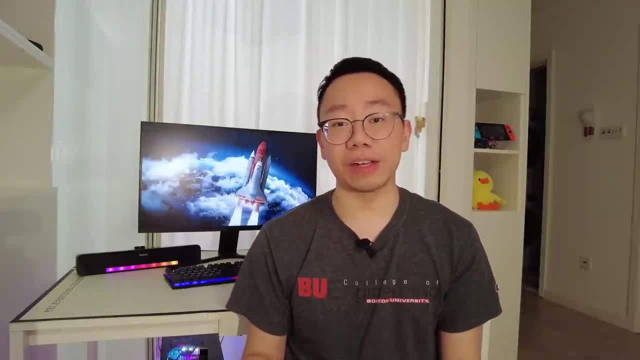 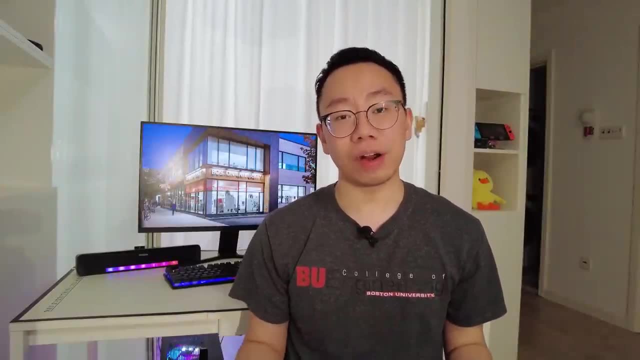 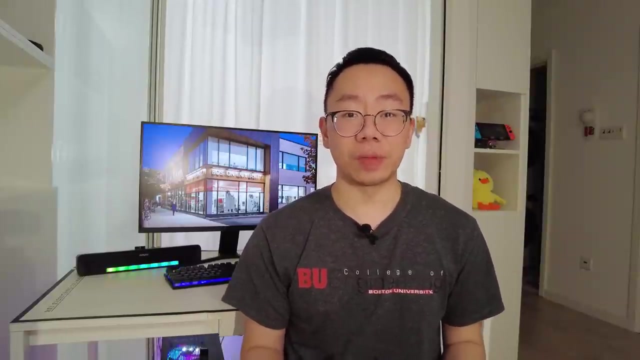 monte carlo, Understand the pros and cons of each and try doing a calculation using excel or 3dcs. Okay, so these are some of the things I would focus on if I could start over and go back to university to relearn the material. By no means is it an exhaustive list, but as an engineer, 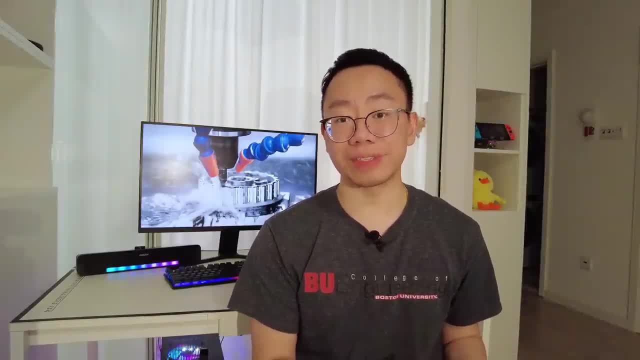 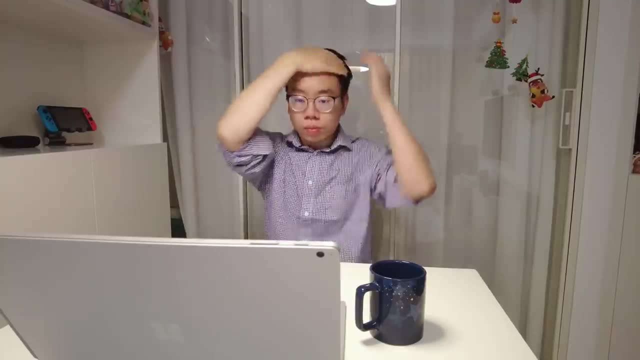 you'll be in a very good spot if you work on understanding the theoretical concepts and developing the practical skills that we just covered. As much as I hate to say this, knowing these things cannot guarantee that you will pass engineering interviews and land your dream job. It will definitely help, but it doesn't. 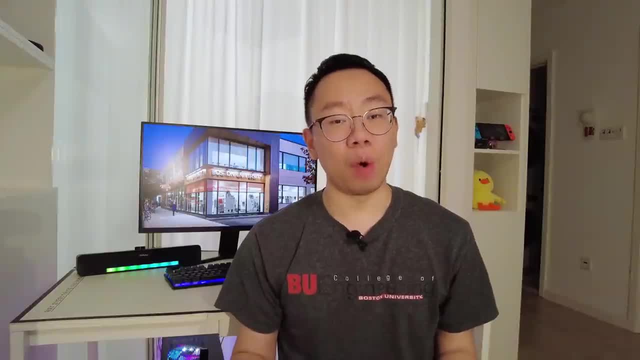 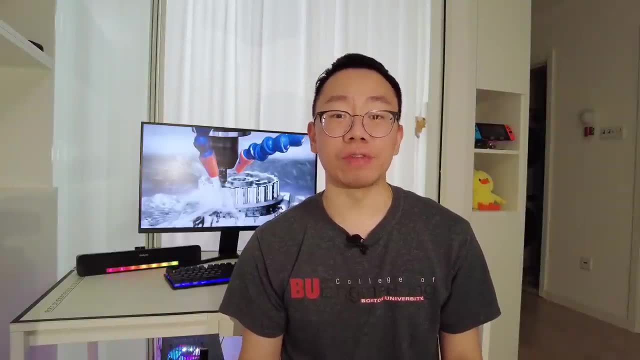 guarantee anything. That's just the hard truth. Now I want every single one of you to land your dream job. so if there's one thing I wish I knew before interviewing for all of these jobs, it is a systematic way to prepare for these interviews. First, I will research everything. 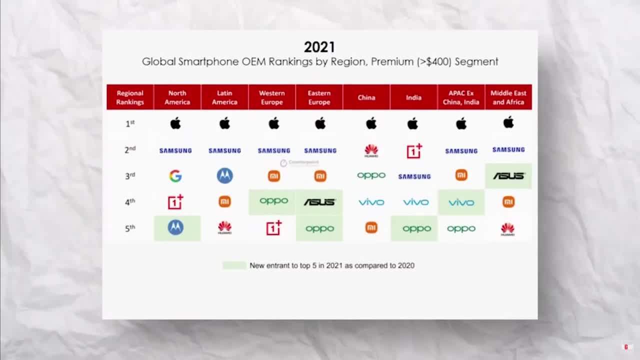 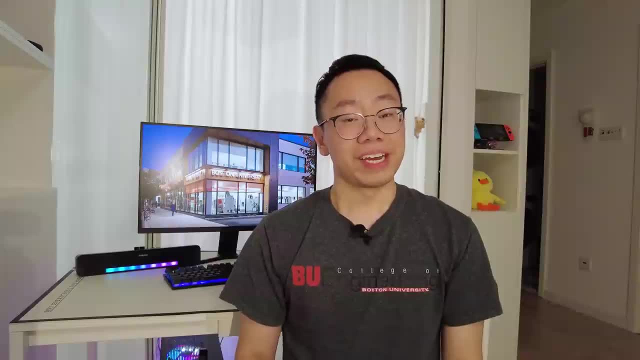 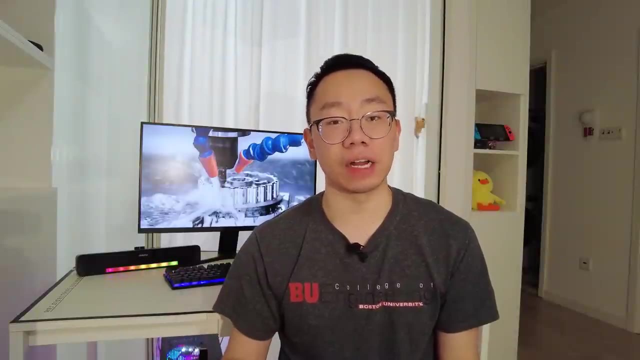 about the company I'm interviewing for Their products editors, history, mission and growth strategy. Second, I will know my resume and job description inside and out, Because engineering managers love to kick off interviews by going through the projects and qualifications listed on your resume before getting into the meat of the. 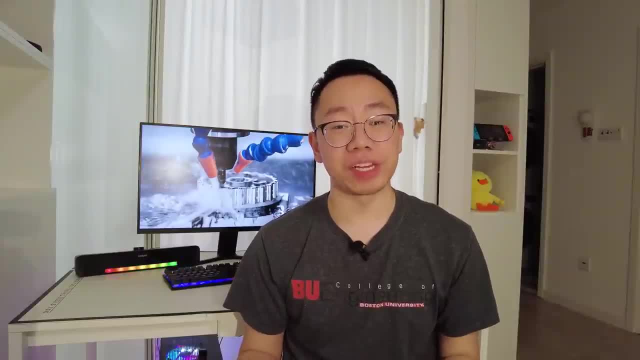 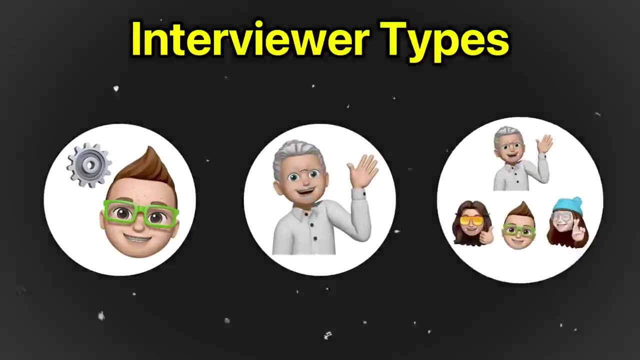 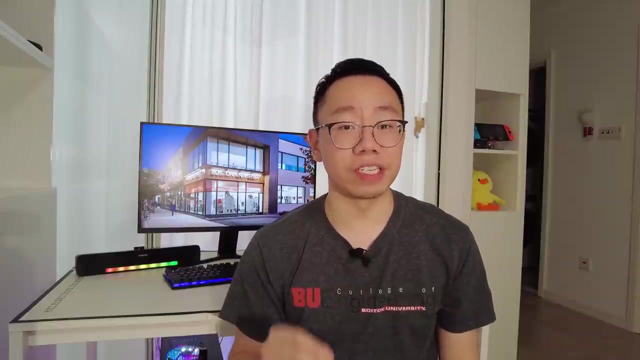 technical questions. Now, the hardest part about mechanical engineering technical interviews is you never know what the interviewer- who could be an engineer, engineering hiring manager or a panel of engineers- will ask. Mechanical engineering is a very broad discipline and technical questions tend to either be very specific or have to do with challenges that the company is currently facing. 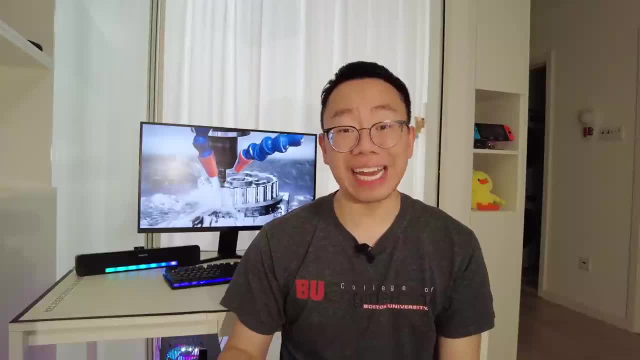 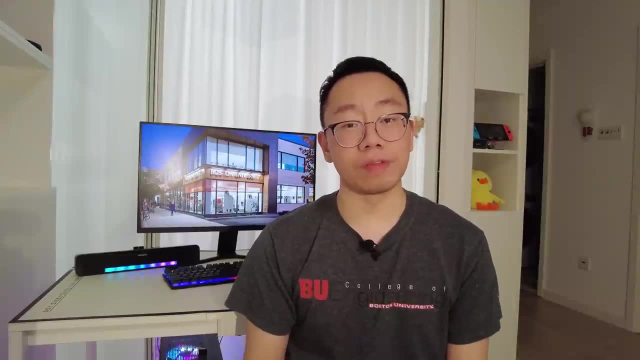 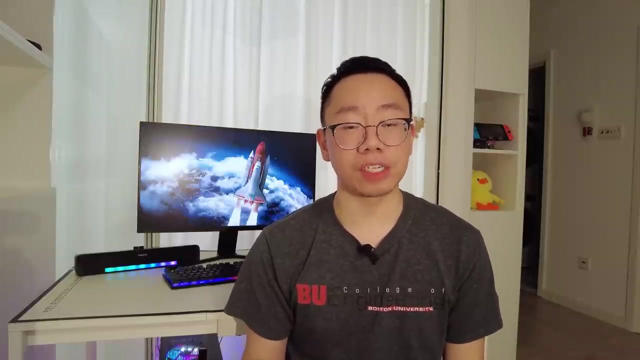 So you would only be able to answer these questions if you've done a ton of technical interviews in the past or worked in industry as an engineer for a year or two. Unlike coding technical interviews, where questions are transparent and available on platforms like Leetcode and AlgoExpert, mechanical engineering questions are wildcard and way harder to prepare. 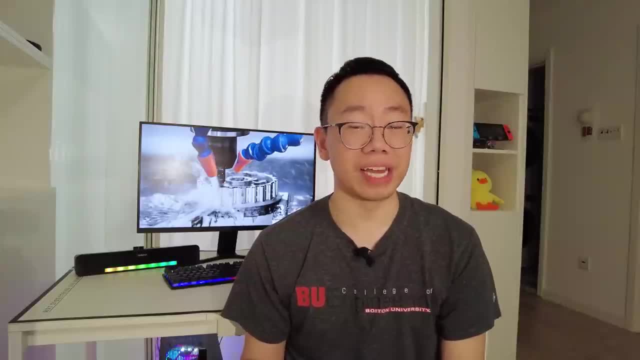 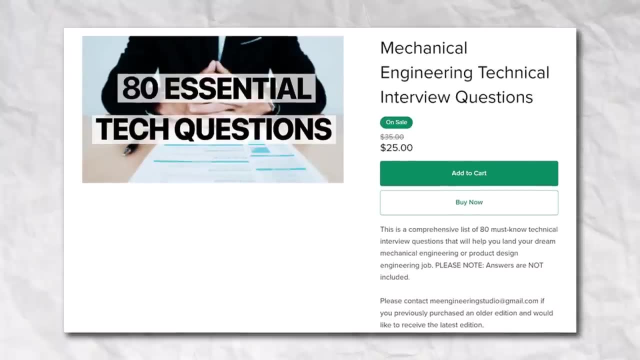 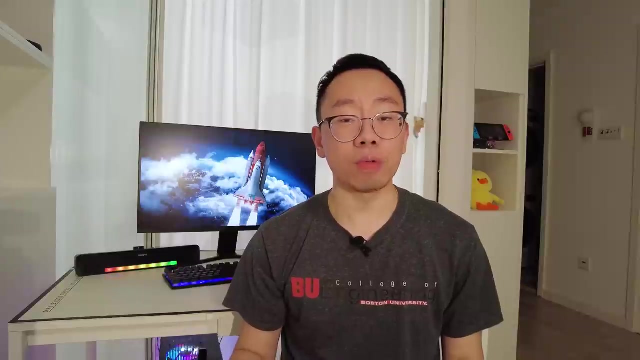 The technical interviews always seem to trip me up as a student in university, so I learn everything the hard way through trial and error. To help you guys out, I put together a list of 80 technical practice questions spanning all areas of mechanical engineering that I think are great to know and hopefully will.